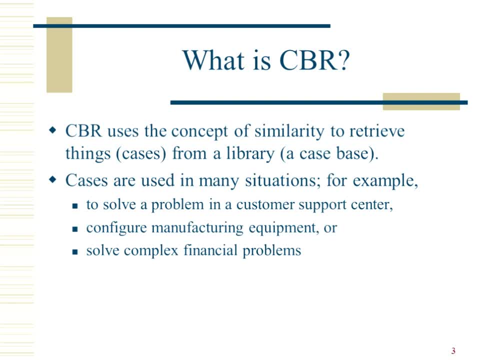 the CBR technique. the main idea behind this technique is that many problems that we face in our lives, they are very similar to the old problems And the solution of those problems can be directly used to solve these new problems. So there is some similarity between the new cases and the old cases. 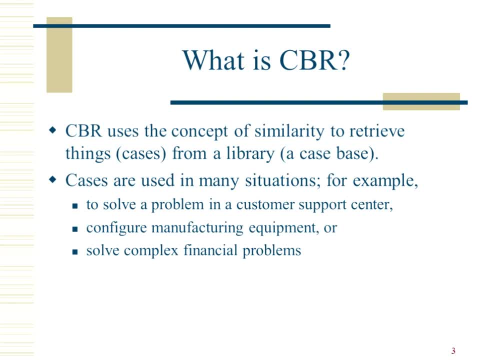 The new problems and the old problems And we can use the solution of those old problems to solve the current new problems. So the cases are used in many situations, For example, to solve a problem in a customer support center To configure manufacturing equipment. 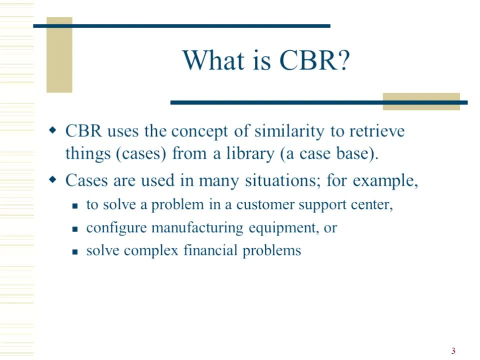 To solve complex financial problems, To diagnose the patient in different diseases, To prescribe certain medicine to them, And so on and so forth. So all of these examples have a certain problem And there is a certain solution. The idea is that if we archive all those solutions, 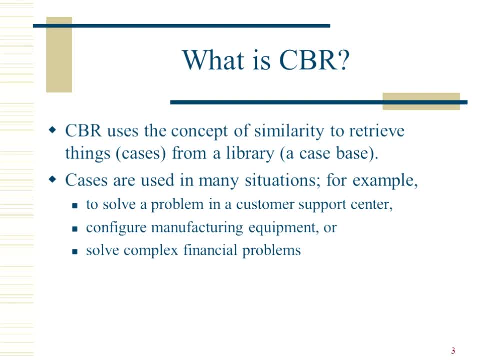 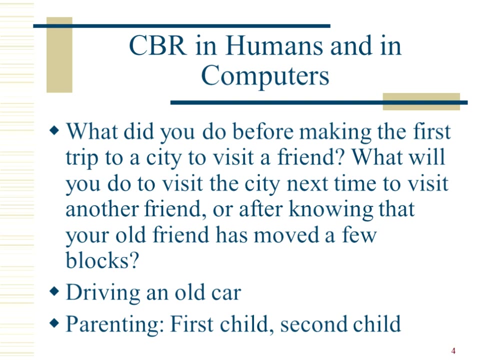 whenever we encounter a new problem, we can find the similarity of the current problem with one of the old problems, or more than one as well, And we can use these solutions to solve the current problem. We use CBR in our daily life quite often. 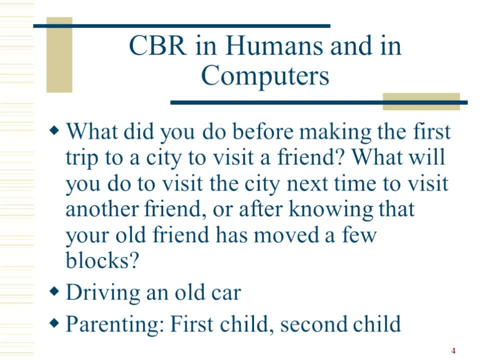 Just to give you a couple of examples. What did you do before making the first trip to a city to visit a friend? So just imagine that if you want to visit a friend, you make a complete plan. You will see the map. You will ask your friend about certain landmarks. 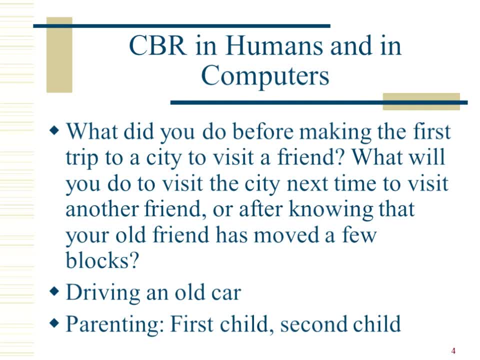 And then you will go there, You will follow certain landmarks And keep navigating. Maybe you will forget a couple of times. Then you will go back and forth and so on and so forth, Until and unless you have reached your destination. Just imagine the second time if you have to go to the same friend. 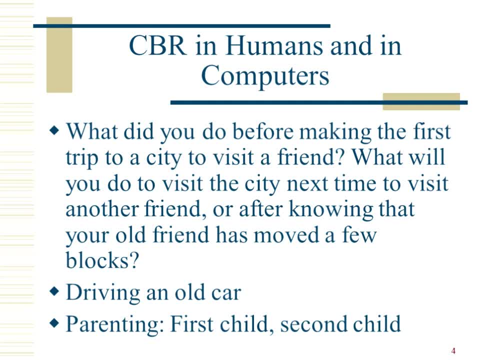 Now you will not have that much difficulty as you had in the first time. Nowadays we have navigators And sometimes navigators. they are quite helpful, But even then sometimes they miss you. But anyway, the concept is that the second time 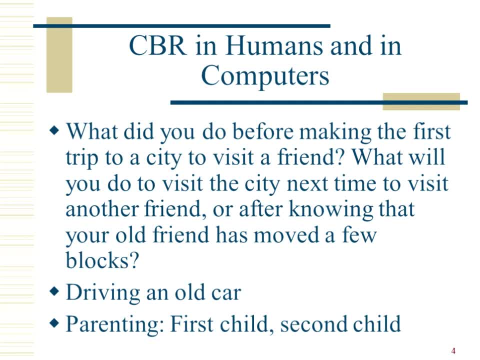 if you want to visit the same location, it will be easier to reach that point based on the steps you had navigated in the last visit. And just imagine that if the same friend has moved to another place in that same area, in the same district, in the same location, 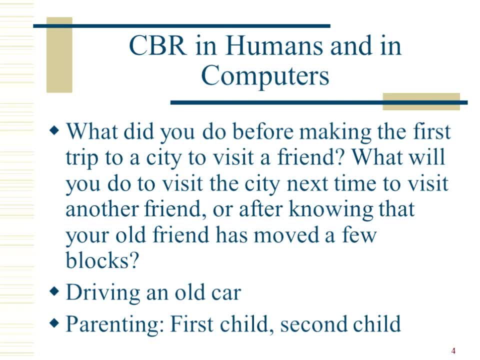 maybe just a couple of blocks away. Now you can reuse the entire solution of the previous visit And from that point onward you can locate the new location quite easily. So this is one example of case-based reasoning. You had a case. The first visit was one case. 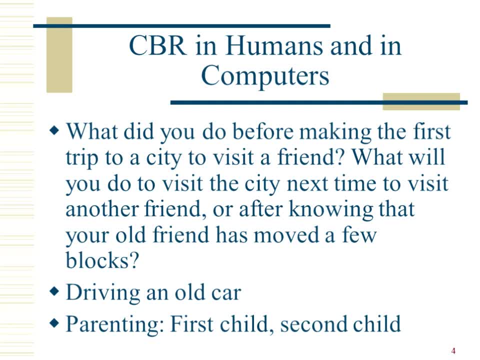 And then you use the solution to solve the new case of a new location, Similarly, driving an old car. Let's say you buy a used car And the first time when you face a problem you panic a lot, But the second time when you face the same problem, 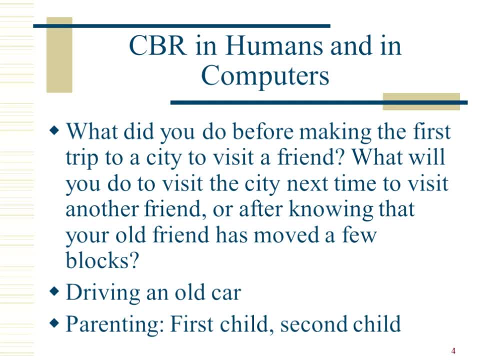 you will know, okay, this car misbehaves in this particular way. This is the trick, this is the tip that I can use to solve the problem next time And after a few months. now you know about ins and outs of the entire car. 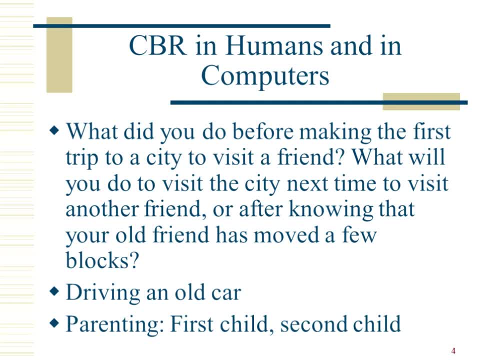 And whenever you face any problem, you can use the same information to sort it out. Similarly, taking the example of parenting, We all know- those of us who are already parents- that raising the first child is quite a challenging task. You are learning many things. 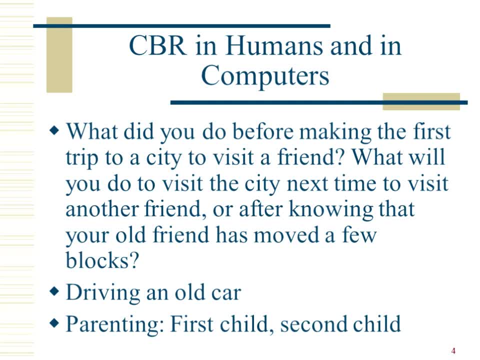 Many things are new for you, But when you have a second child, you reuse the same experience For many times. you contact your parents or grandparents. They guide you. They guide you in many aspects. There are many things which are common in the newborn. 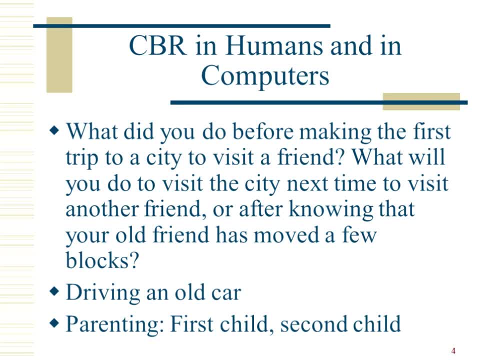 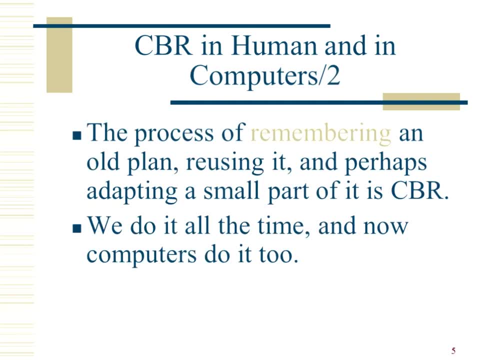 And you can reuse the experience to solve these problems. So these are many examples of using CBR in our daily lives. So the process, the core concept, is that we remember an old plan and we reuse it whenever we face a similar situation. You might not face the same situation again. 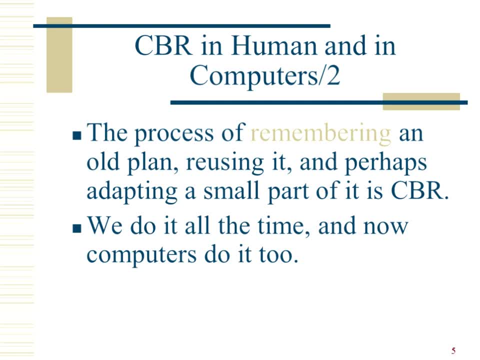 If you do face the same situation, that's good. That's well and good. We can reuse exactly the same plan, But many times we may have to adapt some part of the previous solution And we can come up with a solution to the new problem. 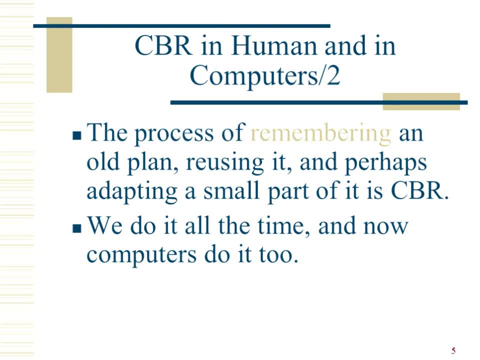 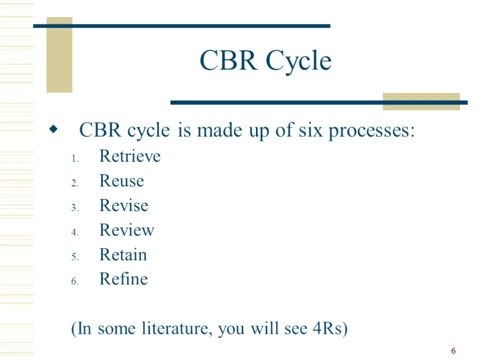 So we have been doing it in our entire life, And now the computers, they also do it in the form of one technique which is called case-based review. So these are the six processes, or six changes, six steps in the CBR process. 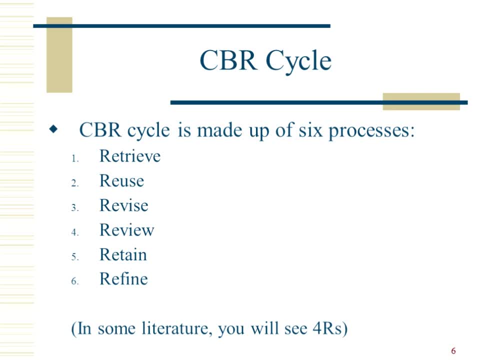 We retrieve the old cases, We reuse them, We revise them to adapt to the new problem, We review them to learn something new- We'll talk about it in a second- And we retain the solution so that it can help us in solving the next problems in the future. 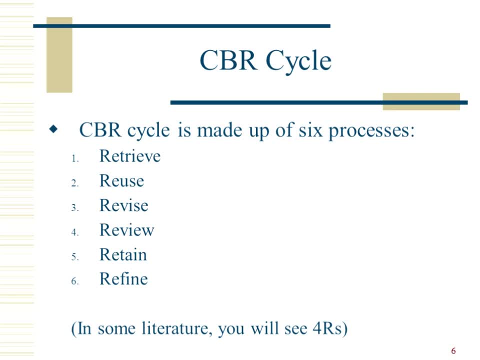 And we also refine our case-based to always keep it updated. In some literature you will see four R's, Here we have six, But in some techniques, in some literature you'll find four R's that review and refine. They are not mentioned in some processes. 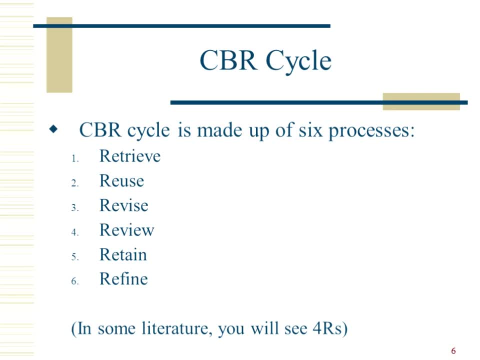 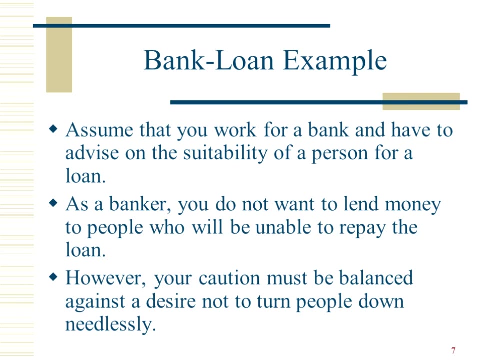 But anyway, in all the cases, the basic concept remains the same: to renew the solution of our problems to be able to solve the new problems. So let's discuss details of all these six phases. Taking the example of bank loans, we had also discussed it briefly in the previous course. 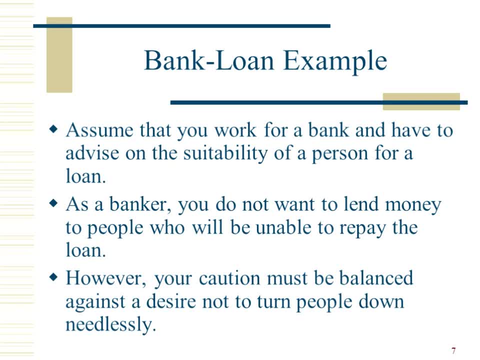 It seems that you work for a bank and have to advise on the availability of a person for loans. Now, many people they submit applications to apply for loans But you cannot approve. you cannot give loans to everybody And at the same time you cannot refuse everyone as well. 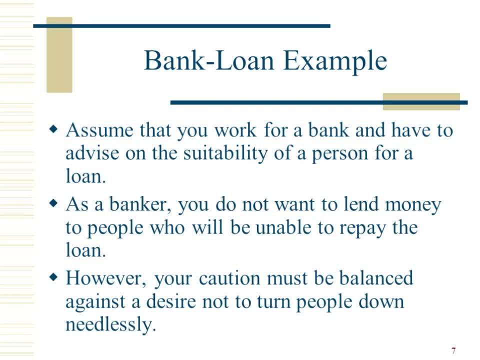 So, as a banker, you want to lend the money to only those people who will be able to buy, who will be able to pay back all the amount. So you do not want to lend money to anyone who will not be able to pay back. 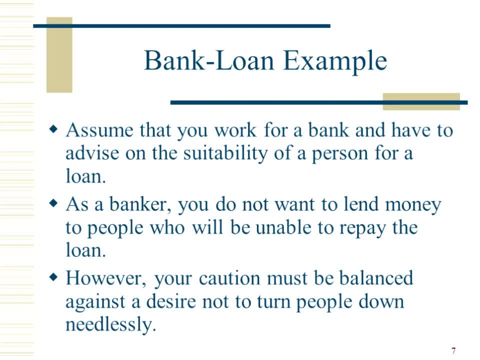 And similarly, you also do not want to refuse everybody right. So you need to strike a balance, Because the banks, they make money from these loans and they lose money if a customer is unable to pay back. So you have to strike a balance. 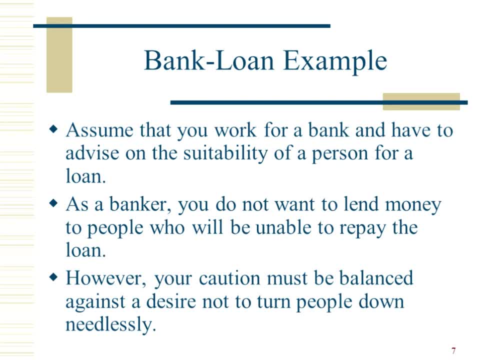 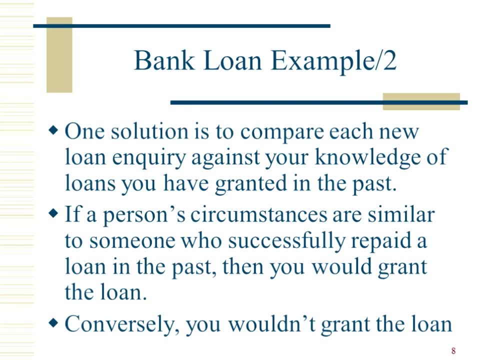 to filter out those people who will not be able to pay back and to encourage those people who will be able to pay back the loan. So whenever a new customer applies for a loan, one simple solution is that you compare this current application with your knowledge of the loan that you have granted in the past. 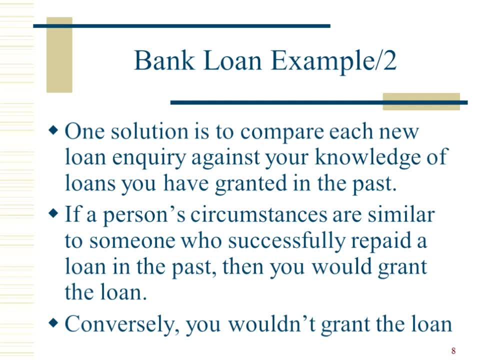 Let's say you are working in that bank for the last five years and in these five years you came across several applicants. Many of them were able to pay back and many were unable to pay back their loans. So if this new customer's situation 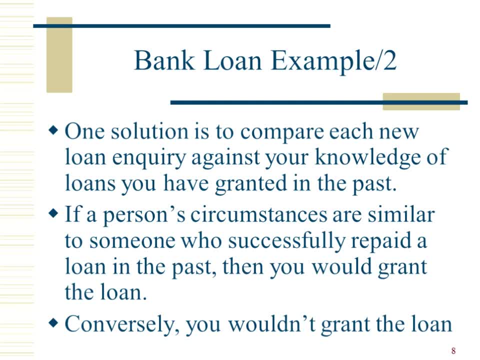 the circumstances of this new customer. they are similar to a person who was able to successfully pay back, then you grant the loan. Otherwise, if his or her situation is more similar to someone who is not able to pay back the money, then you will not grant the loan. 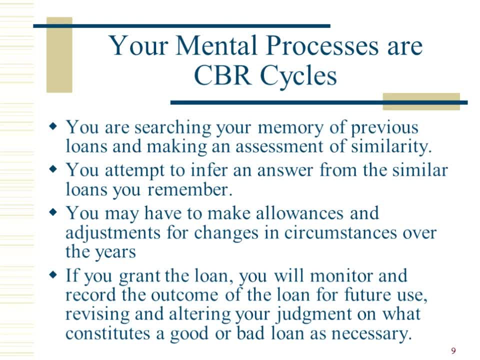 Right, It's a very simple concept. So what you are doing, you are searching for memory of previous loans and making an assessment of similarity. You are scratching your memory, You are trying to recall the cases and trying to find a similarity and then, based on this similarity, 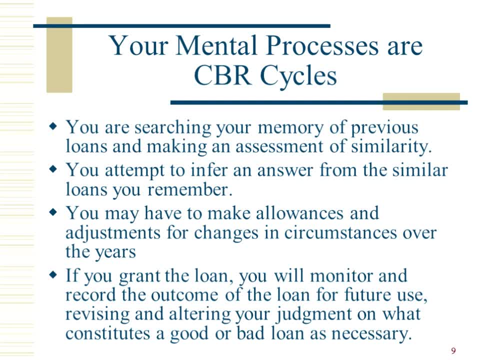 you make a decision, you make a choice, So you attempt to infer an answer from a similar loan and you may have to make allowances and adjustments for changes in circumstances over the years. What do we mean by this? Let's say you granted a loan in 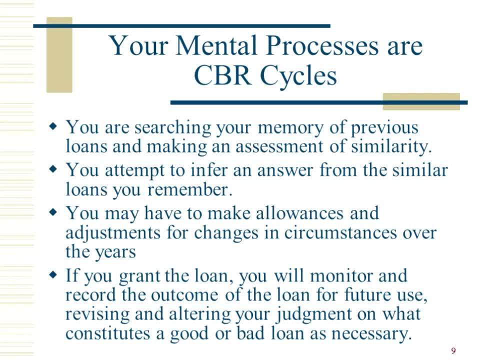 let's say, ten years ago, and you know what was the income of that person. And today a person is applying for a loan and you also know his or her income. Now you make an adjustment like 20,000 ten years ago. 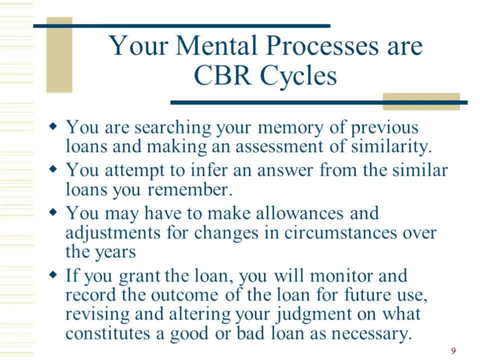 will be equivalent to a salary of, let's say, 25,000 today. Right, So this is a main concept in case-based reasoning: that we try to find the similarity and then we try to make the adjustments, also to use the old solution to solve the current problem. 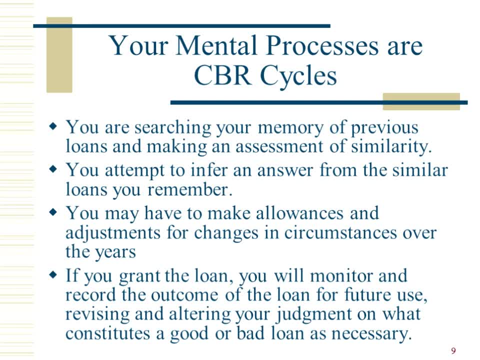 And also, if you grant the loan, you'll monitor and record the outcome of the loan for future use. So now, today, you give a loan to a customer and you will also monitor and when the period expires, you'll be able to tag this new customer. 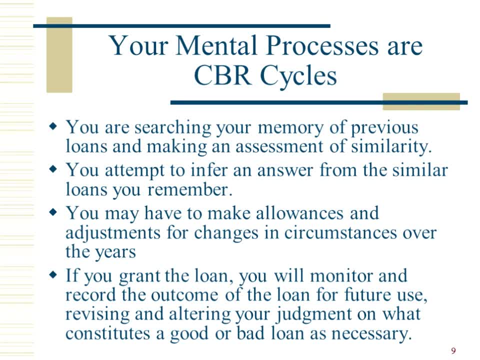 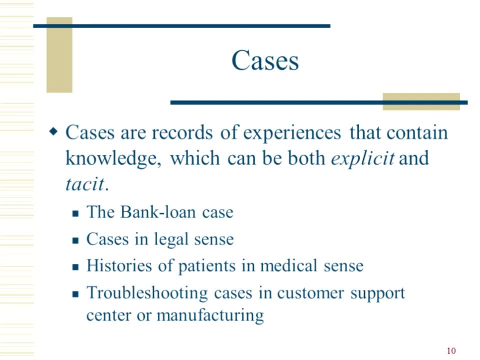 as good or bad, whether he or she was able to pay back or he was not able to pay back the loan. So this is the mental process of EDR cycles, Thank you. So the heart of case-based reasoning is cases In simple words. 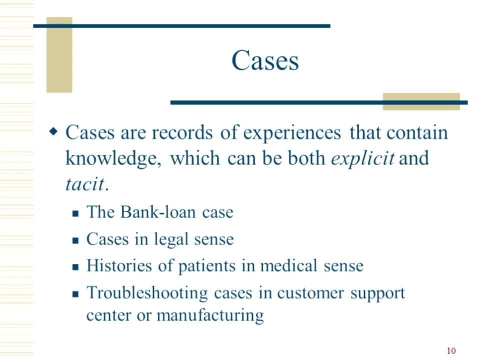 cases are records of experiences that contain knowledge which can be both explicit and explicit. So all these customers that you have dealt with throughout your experience in the bank, they are all cases And in every domain we have cases. For example, we just discussed banking on case. 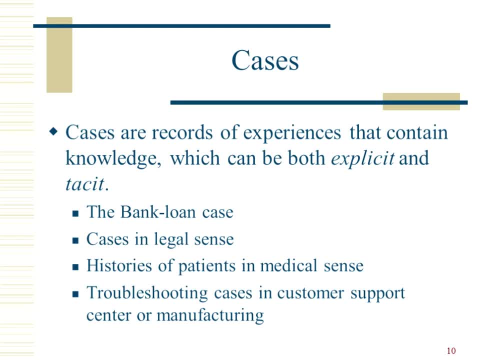 We have cases in the legal sense In the courts. there are cases There are disputes between the people. There are cases Similarly in medical domain, the historical record of the patients. there are the cases Similarly for troubleshooting anything. 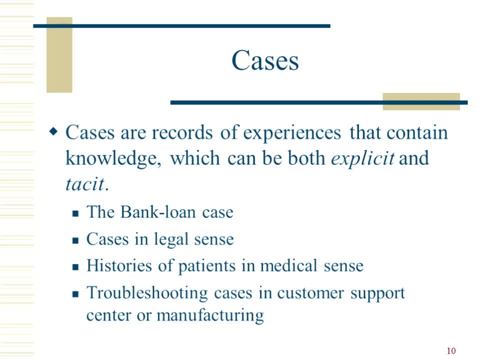 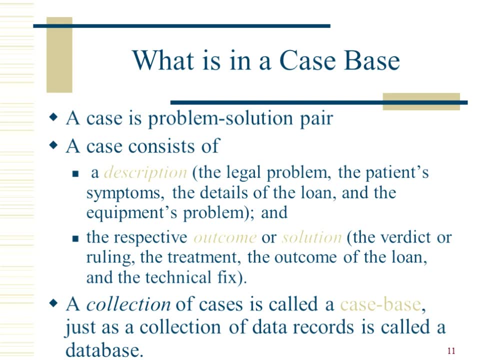 this troubleshooting experience are the cases. So every case contains two things: It's a pair of problems and the solution to that problem. So a case consists of a description of the problem, like the legal problem, like the patient for patient, the patient's symptom. 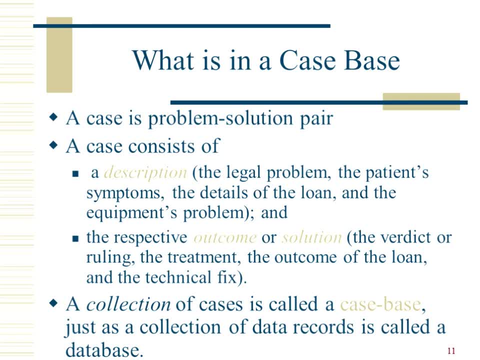 For the loan, let's say the income of the person, the monthly installment that he had to pay back, his background, and so on and so forth. The equipment problem. so it will consist of a description of that problem. We have certain attributes. 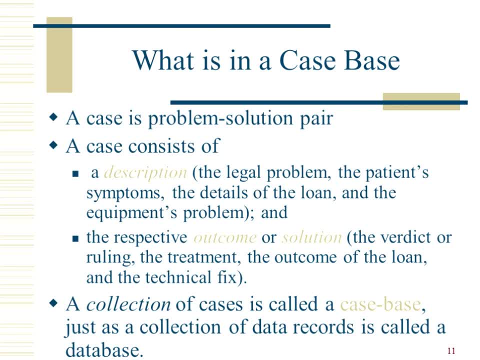 We have certain features, a feature set that is used to describe the problem, And the second thing is the outcome or solution: the ruling in the legal problem, the treatment for patient problem, the outcome of the loan for loan problem and the technical fit for an outcome. 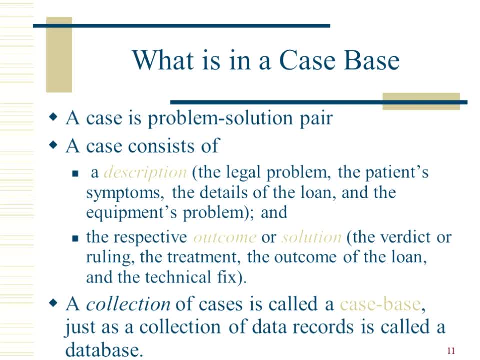 And the third thing is the outcome of the loan for loan problem and the technical fit for an equipment troubleshooting problem. So a collection of the cases is called a case base, Case base, Just like a collection of data cards is called a data base. 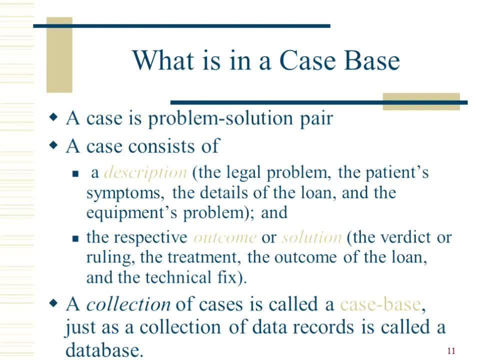 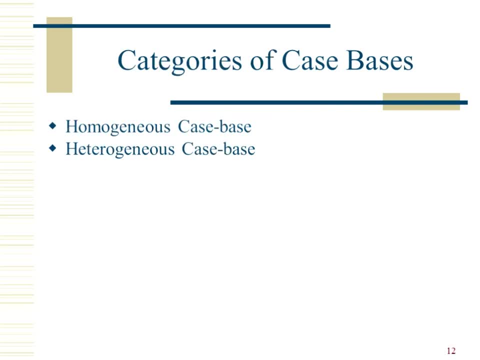 So in a case base we will have several problem-solution pairs in which we describe all the problems and we give solution or outcome of those problems. There are two categories of case bases. We have homogeneous case base and we may have heterogeneous case base. 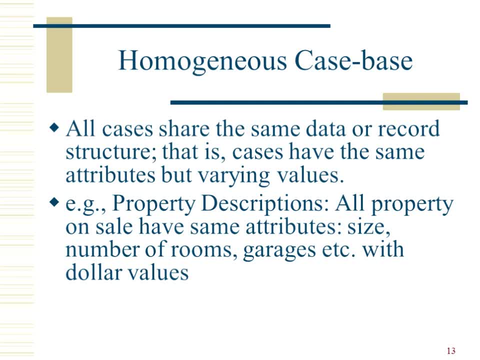 What is a homogeneous case base? In a homogeneous case base, all cases share the same data or record structure. The cases have the same attributes. Of course, the values of the attributes will be different for every case. If the values are all the same. 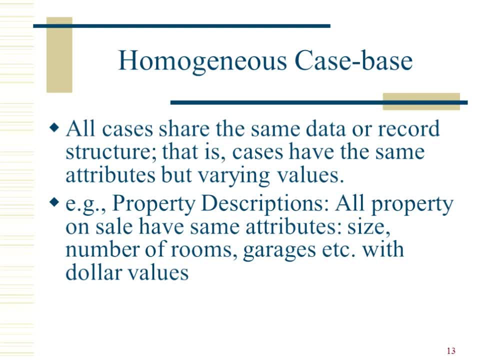 then there's no point in having different cases. But the attributes, the features of those cases, they are same, The structure is same. For example, let's say we talk about a loan case, So let's say the features are the total amount of loan granted. 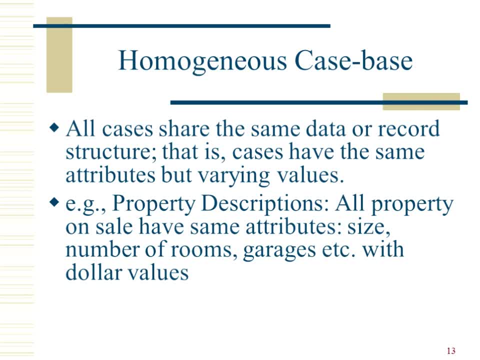 the, let's say, age of the person, let's say the income of the person, let's say the industry or the job of that person, and so on and so forth. So all these are the features of this case, For every loan application. 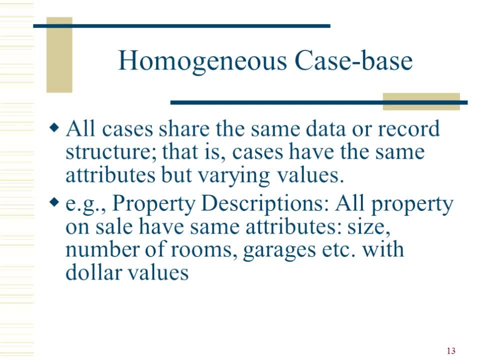 every applicant will have a value for each of these features, but the feature set will remain the same. Okay, For example. another example on the slide is the property description. Let's say we are working for we are making that case base for property dealers. 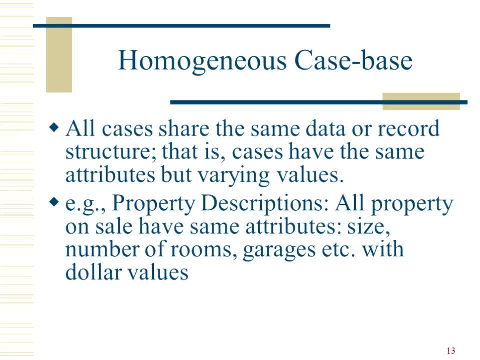 who buy and sell the houses and pieces of land. So all the properties. they have same attributes, Like every house has a size, number of rooms, garage, the area, price and so on and so forth. So the values are different. 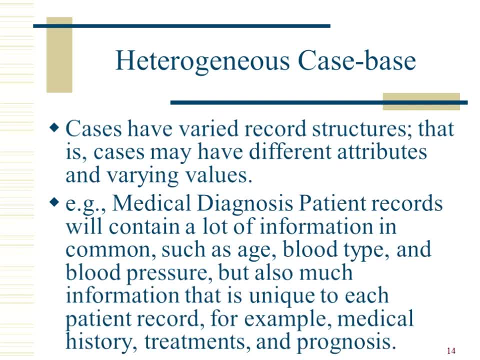 but the feature set is same for all the cases. On the other hand, for heterogeneous cases, the cases have varied record structure. The cases may have different attributes and different values, of course. For example, let's talk about medical diagnosis Now. 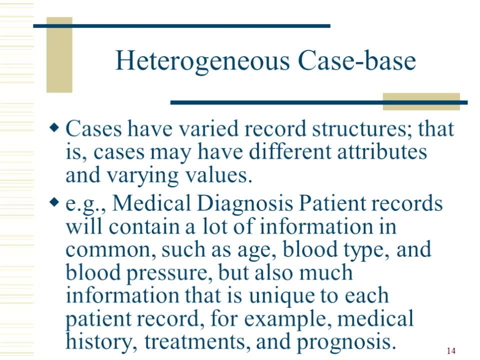 every patient will have unique disease and every patient will have unique tests. So maybe for one person we are taking the test of, let's say, a kidney function test, let's say creatinine level and other kidney function, For another, 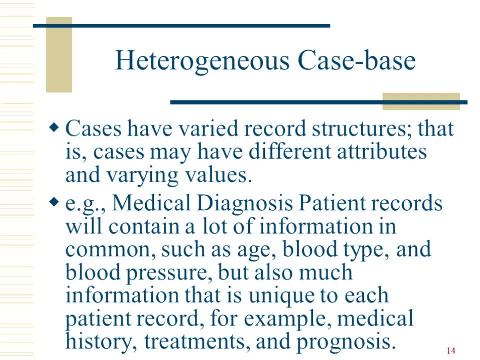 maybe the complete blood count and other blood tests. Maybe for some we are making x-rays, For some maybe CT scans, For another maybe MRI and so on and so forth. So you know that there are hundreds of different conditions. There are hundreds of symptoms. 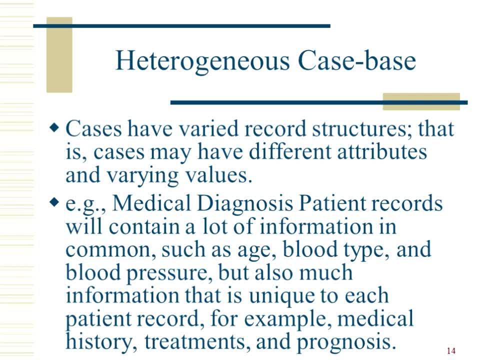 There are hundreds of medical tests, There are a large number of different diagnosis, and then the medicine that we prescribe, and so on and so forth. So you see, every patient will have a different set of attributes to define his or her own unique case. 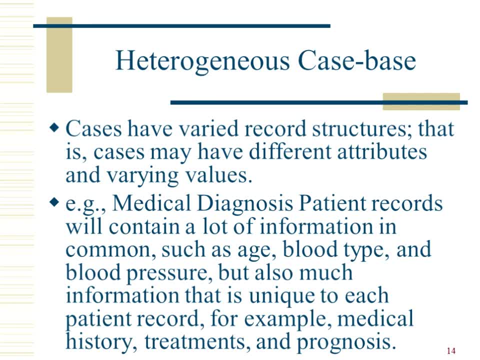 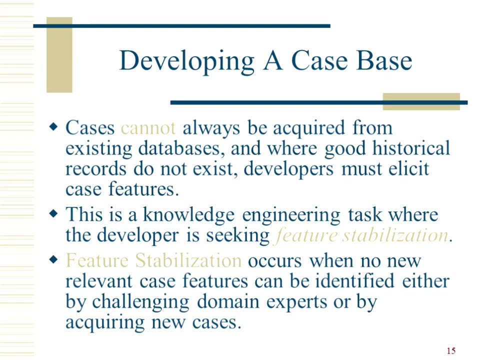 So these cases will be heterogeneous. Every case may have different attributes and, of course, the values of those attributes are also different. Now coming to designing a case-based system. first of all, we'll talk about the case-based development: how we develop a case-based. 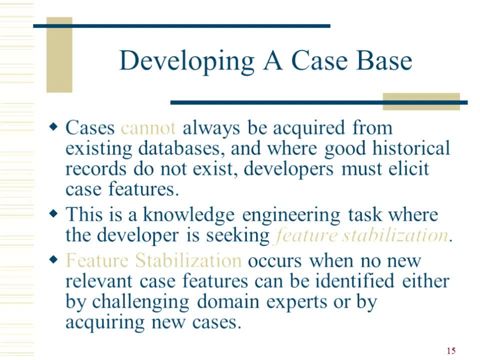 Cases cannot be defined. Cases cannot be defined. Cases cannot always be acquired from existing databases. Well, if we have a database from which we can acquire cases, that's very good. That's very easy. It makes the life of a developer quite easy. 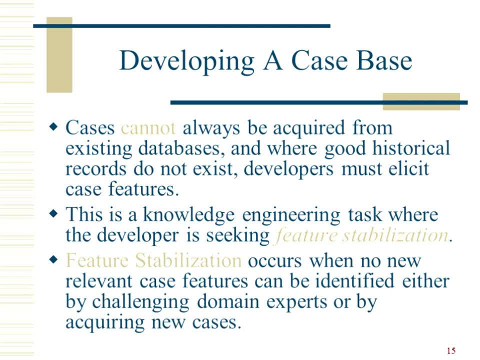 But it is not always possible to acquire all the cases just by pulling the information from a database, and the good historical records do not exist. Developers have to enlist it, They have to develop the case and the case features. So this is a knowledge engineering task. 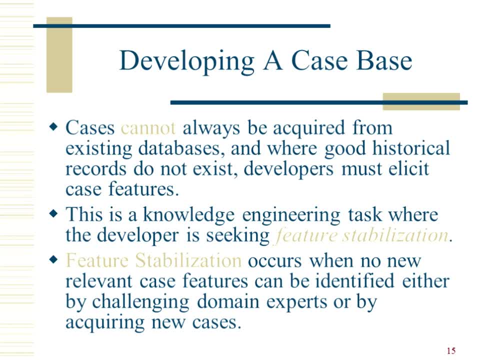 and the developer will try to stabilize the features. We call it feature stabilization. What does it mean? It means that no relevant case feature we have achieved feature stabilization when no new relevant case feature can be identified When we have captured all the case features. 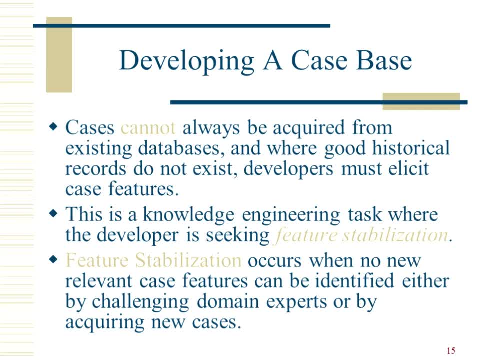 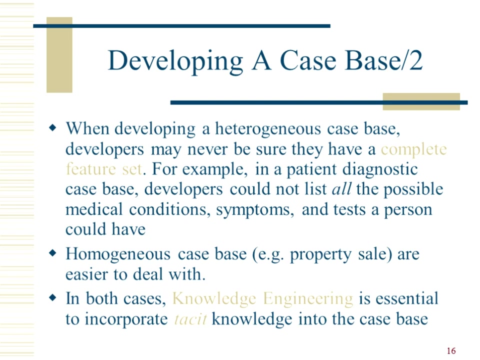 or attributes that describe each and every possible case. So we do not expect any case with a feature which is outside our list of attributes that we have already gathered. Of course, it is not easy for heterogeneous cases When we are developing heterogeneous cases. 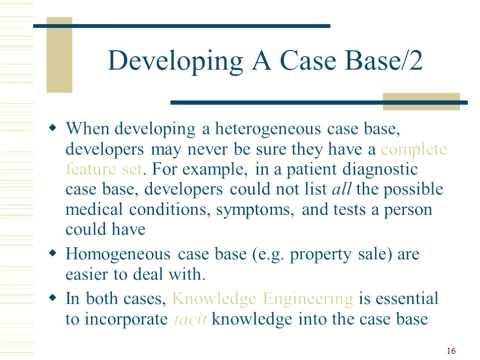 we can never be sure that they have a complete feature set. For example, in patient diagnostic cases, developers could not list all possible medical conditions, all possible symptoms, all possible tests, medical tests, all possible kind of treatment and medicine. So for heterogeneous. 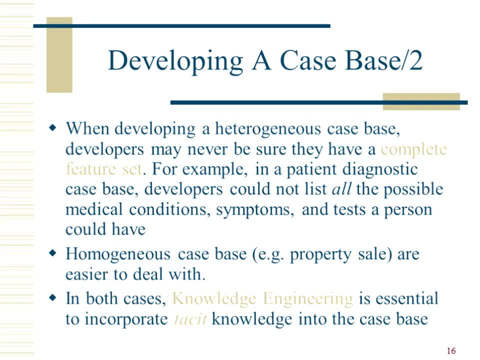 it is a very, very challenging task and you can never be sure that you have a complete feature set. However, for homogeneous cases, it is easy to deal with it and a knowledge engineer, in consultation with an expert, will try to identify and narrow down. 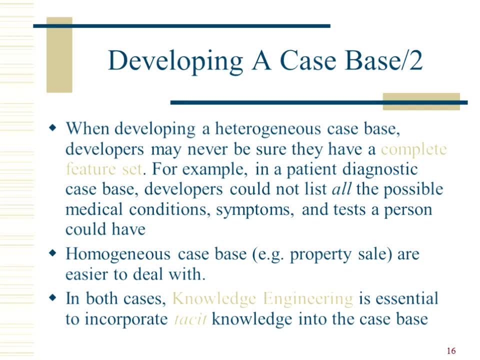 all the cases, that capture all possible features or the attributes that will describe each and every possible case in the domain. In both cases, whether we have heterogeneous or homogeneous case base, it is also essential to incorporate the case knowledge into the case base We have been learning throughout this course. 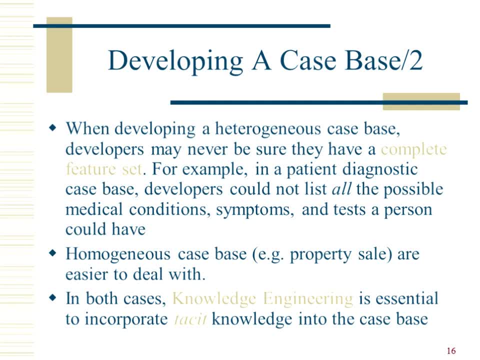 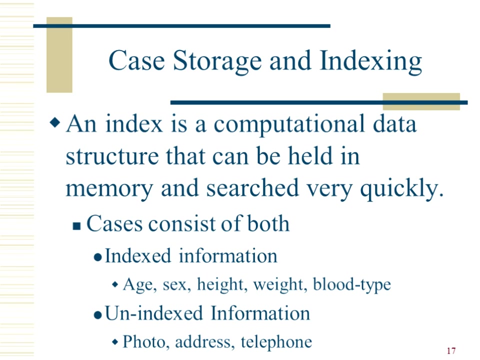 that case knowledge is also very important, and when we talk about case-based reasoning, it is also essential to merge the explicit knowledge with the basic knowledge. How we do it, inshallah, we will talk about it in the coming slides. Now, in developing a case base, 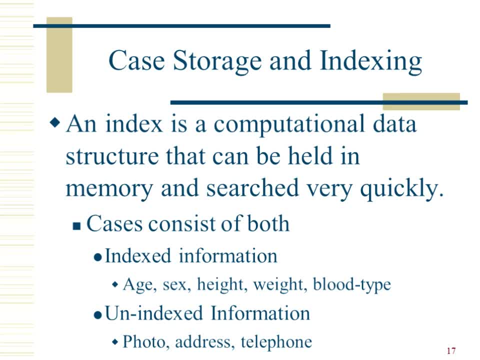 one of the most important things is the index. We had discussed in the last course as well that we need to identify features and we need to index them for quick retrieval, searching and matching with the new case. So all of you are well familiar with the indexes. 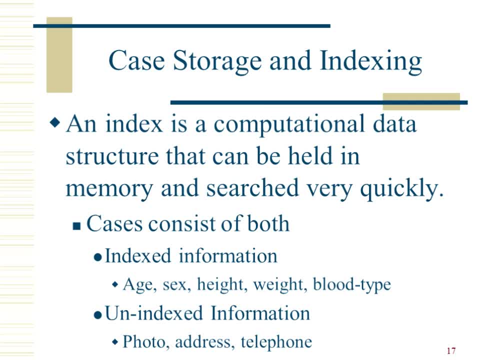 I'm sure you have studied in detail in the advanced database course. An index is a computational data structure that can be read in memory and searched very quickly. So an index resides in the main memory and it is used to quickly search for the relevant case. 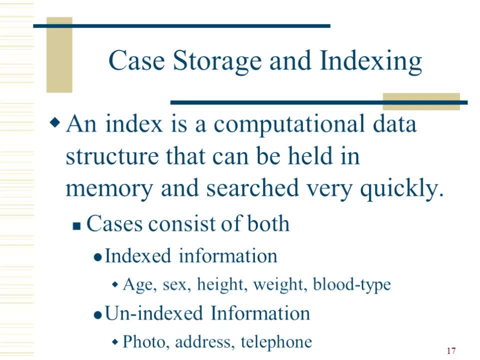 Now in the case base. in the cases, we may have both kind of features. We may have indexed features and we may have some features which are not indexed, unindexed. The indexed information is the one which helps us in solving the problem. 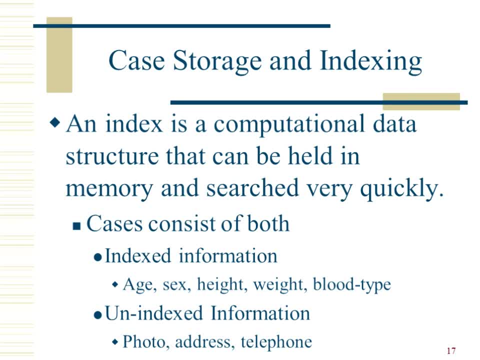 But there are certain features which cannot really help us in solving the problem. They can be used for identifying, for identification or for other purposes, But they do not really help us in solving the problem. For example, here we have a few examples of indexed and unindexed information. 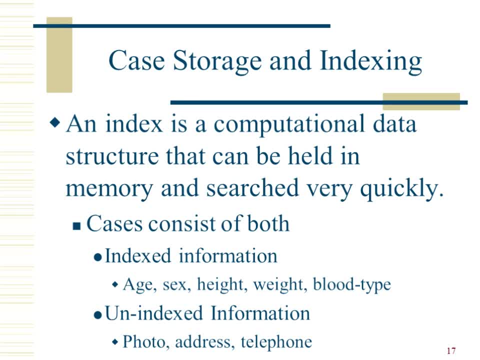 like age, the gender, height, weight, lifetime, All these features, they help us in solving the problem. But a photo, address, telephone number, name of a person, these things they do not help in solving the problem, So they will not be indexed. 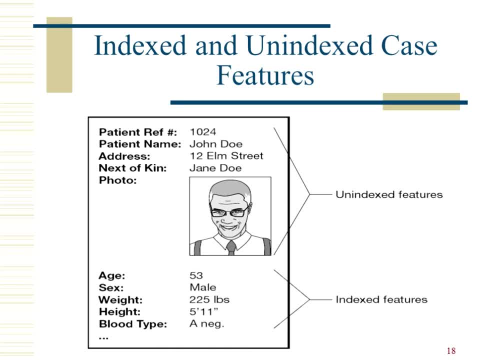 They need to be indexed. So let's say, here we have a case, a patient history, a patient information. So on the top you can see some of the information: identification information of the person, like the reference number, the name. 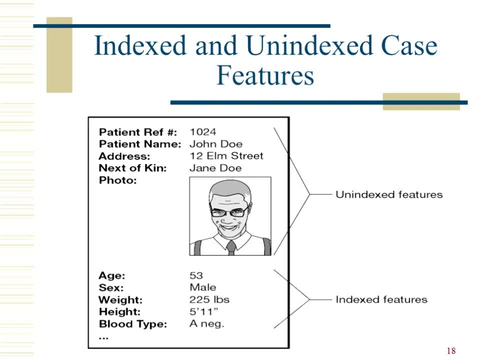 address next to skin name and photo. So all these features, they will be unindexed. They do not help us in solving the problem. For example, in the medical diagnosis of a person, a patient's name does not have any impact on his disease. 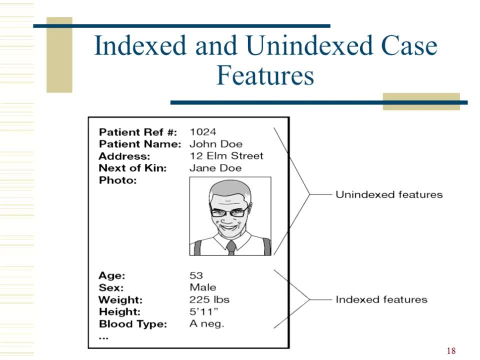 his address and the photograph. they do not have any impact. However, the second set of features: the age, the gender, weight, height, blood type and so on and so forth. they may help us in solving the problem. So these features will be indexed. 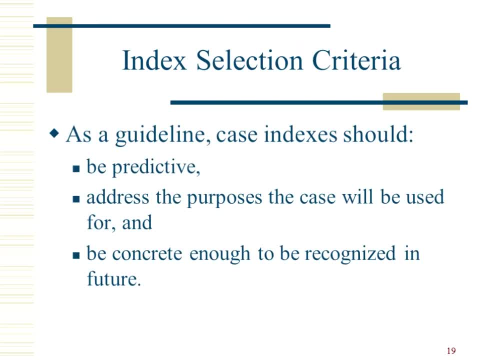 and the above set of features will not be indexed. So the criteria for index selection as a guideline, the case indexes should be predictive. This is one of the most important things that the features. they should help you in predicting or in solving the case. 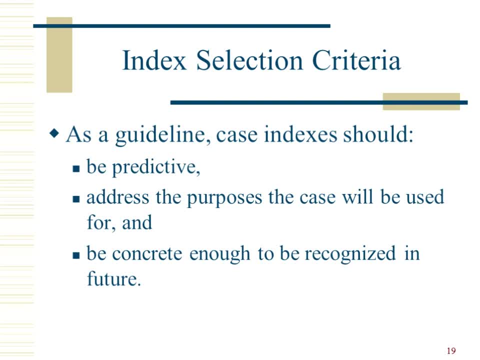 If they do not help. like a name of person, it does not have any impact on the patient's disease or the diagnosis and we do not need to index it. It does not predict. it is not a predictive variable. The indexes should address the purpose. 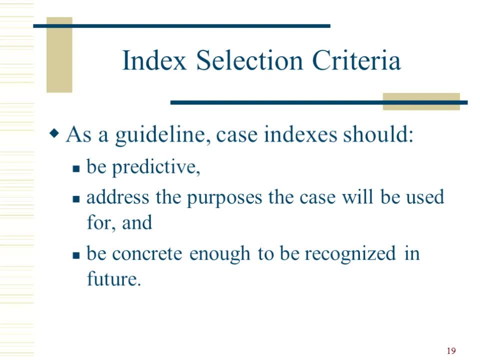 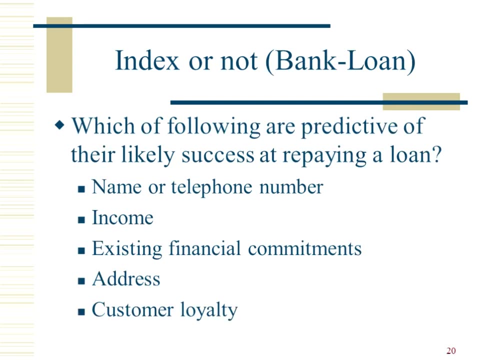 the case will be used for. They should serve the purpose. They should help you in solving the problem. They should be complete enough to be a recognising feature. They should help you in recognising, searching and matching a case with any other case. 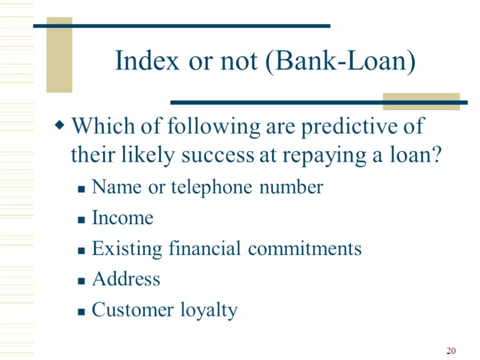 For example, talking about bank loans. here we have a few features and you can easily see or decide which features should be indexed and which should not be. Like name or telephone number, Well, a person's name should not have any impact on his capacity to repay a loan. 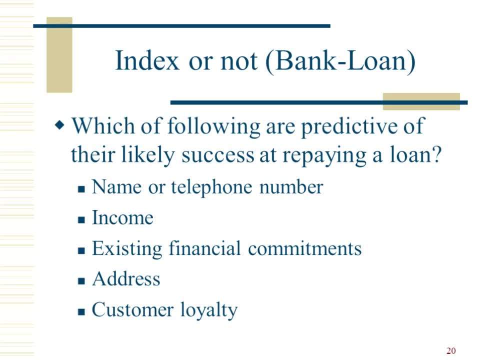 so it should not be indexed. Income should definitely be indexed. The existing financial commitments, of course. If you have any financial commitments, you have taken a loan, you have already taken another loan or you have other commitments, your credit history- these things have impact on your ability. 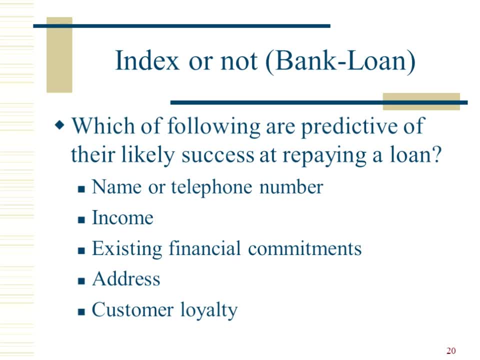 to pay back a loan, It should be indexed. However, the address of the person should not be indexed because it doesn't have any impact on his ability to pay back a loan. Customer loyalty may also have an impact on paying back a loan. 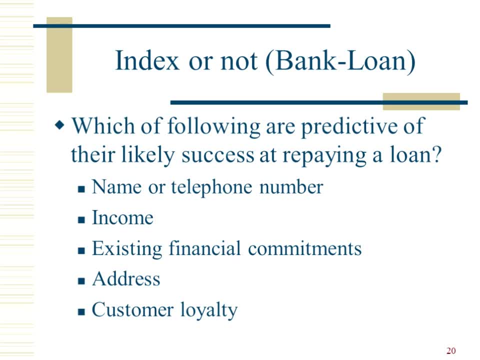 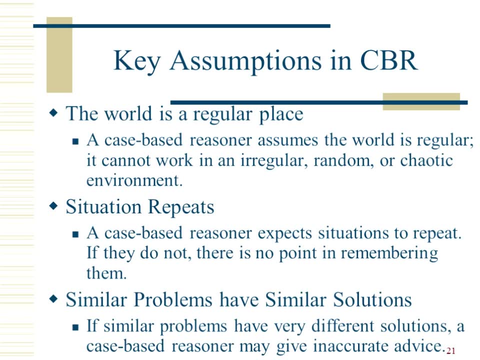 So it's quite obvious that name, telephone number and address, they should not be indexed for this problem. There are certain assumptions in a case-based, in case-based reasoning technique and they should hold for a problem to be able for case-based reasoning. Otherwise, we may not use case-based reasoning. 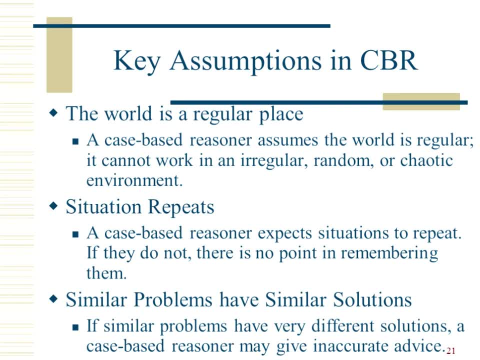 if, for a particular situation, this criteria does not hold. The first thing is: the first assumption is that the word is a regular place. So a case-based reasoning assumes that we are working in a regular domain, In any domain which is chaotic, irregular, random, 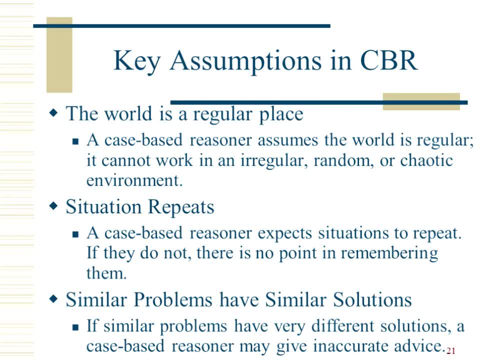 in which you cannot make predictions. you cannot use the case-based reasoning problem. So case-based reasoning assumes that the word is a regular place. It can be only applied for the domain in which the problems are regular, For random kind of problem, for chaotic kind of environment. 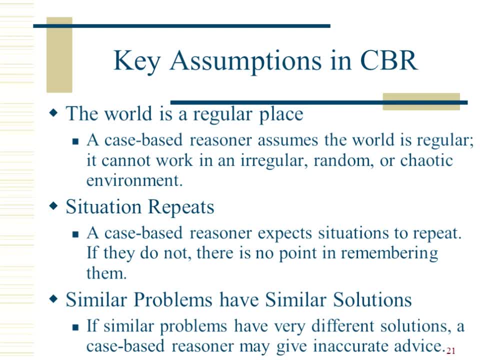 the case-based reasoning will not work. Situation repeats, So case-based reasoning assumes that the cases repeat. If we have a problem and a solution was applied to that problem. if the same problem occurs again, or a similar problem, the same solution, or a similar solution. 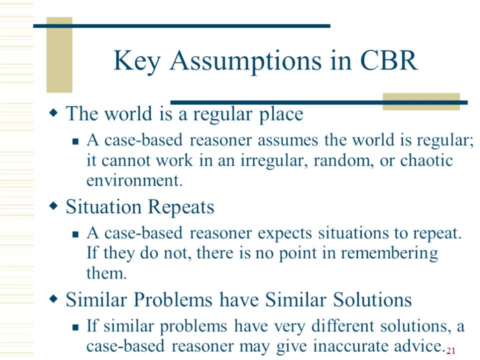 should solve that problem again. So the situations repeat and the solution can be repeated to solve the repeating problems. And the third assumption is: similar problems have similar solutions, That similar problems should have similar solutions. If we use a particular solution to solve a problem, 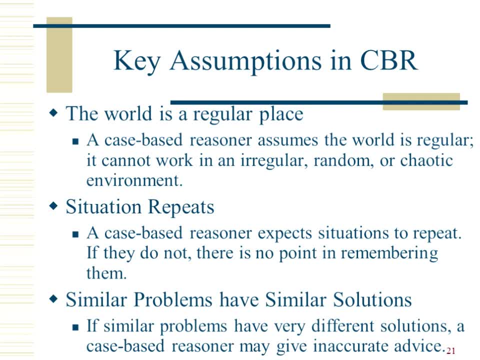 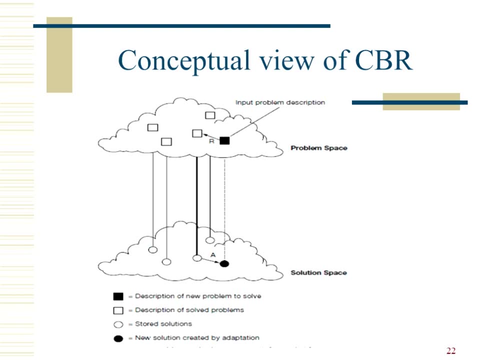 and another problem is quite similar to that. this similar solution should also be able to solve this new problem. So case-based reasoning can only be applied if these conditions hold for a domain. If they do not, then case-based reasoning cannot be applied. 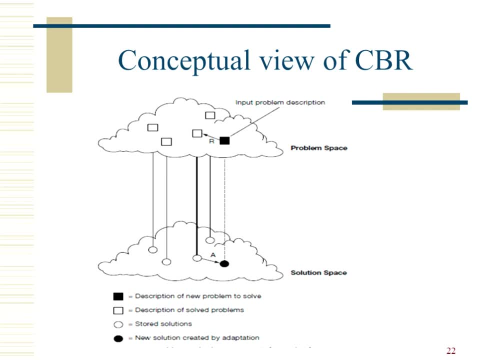 This is a conceptual view of case-based reasoning. On the top you can see the problem space. So we will see how to develop it in Shona soon. So, briefly speaking, problem space contains all the problems. We have kind of plotted all the problems. 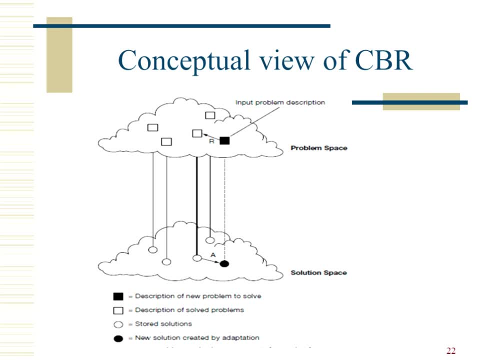 in this problem space, So the empty rectangle. they represent the case space, all the problems that have solutions, And below this you can see the solution space in which these problems, they have corresponding solutions And when a new problem comes. now this filled rectangle that you can see. 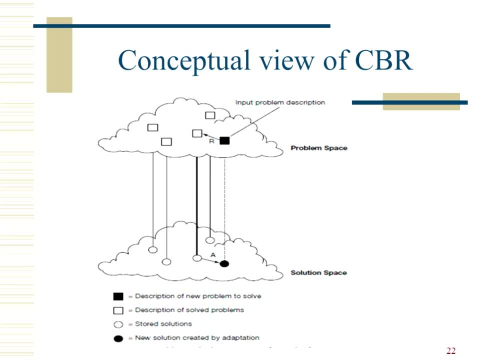 this new problem, like this filled rectangle. this is a new problem and if this problem is similar to an existing problem, now we can reuse the solution of this existing problem to come up with a solution to the new problem. So in the problem space over here, 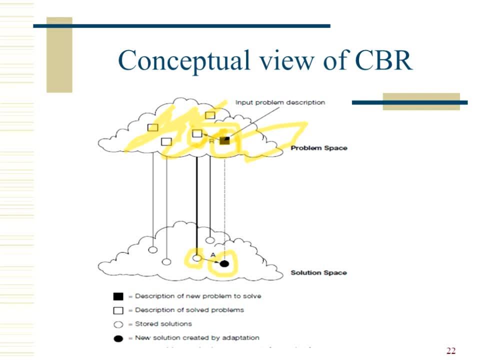 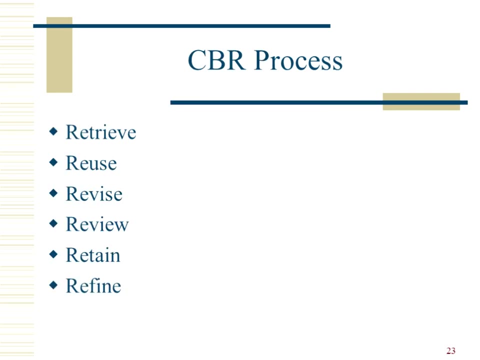 we plot all the cases and whenever a new case comes, we try to find a case which is similar to this problem, and then we use the solution of that problem to find a solution of the new problem. So now let's talk about the six phases. 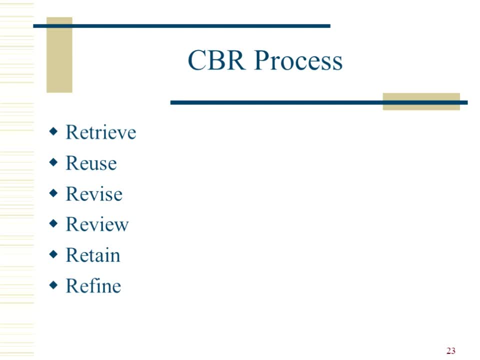 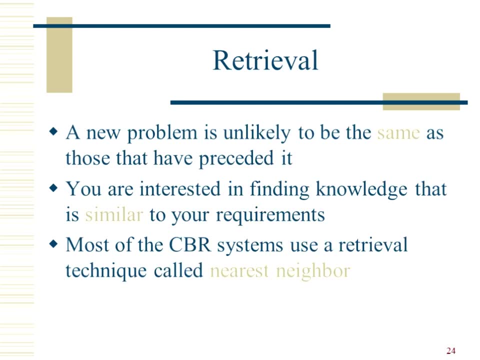 Six steps in the CBR: Retrieve, reuse, revise, review, retain and refine steps. First of all, retrieve. We spend a lot of time on retrieval because it is one of the most important things, So a new problem is unlikely to be the same. 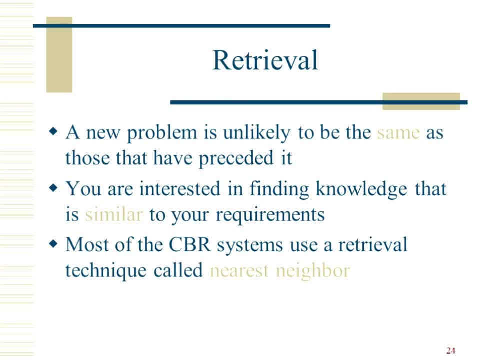 as those that are perceived Well. if we find a problem which is exactly the same as an existing problem, it is very good. It's a good news. We can use the same solution as such to solve the problem, However many times. 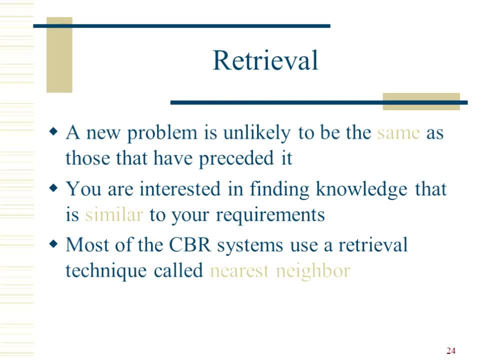 we are interested in finding a similar problem. So many times we find some problems which are similar- not exactly the same, but they are quite similar to the new problem. So to find a similar problem we use a technique which is called the nearest neighbor technique. 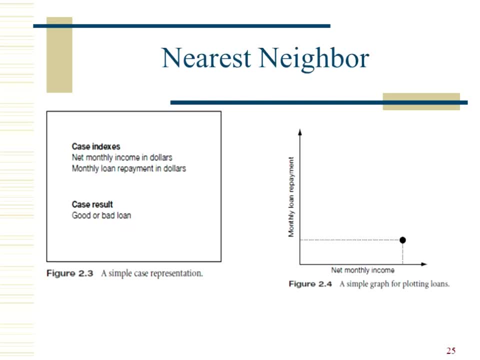 Let's see what is this technique and how it works. Let's take the same example of this loan problem. So let's say we have two features- net monthly income and we have monthly loan repayment in dollars- And the case result is either good or bad loan, right. 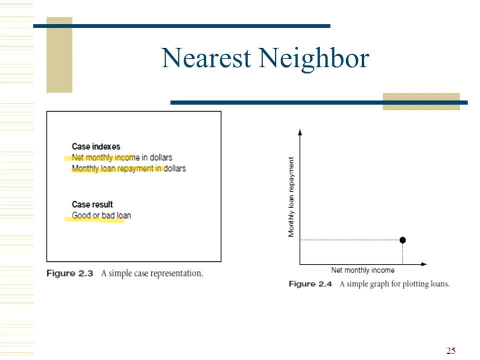 So every user has a net monthly income value in dollars and every user has monthly loan repayment that he or she has to pay back. So in a 2D space we can plot net income on the x-axis and we can plot this. let's say: 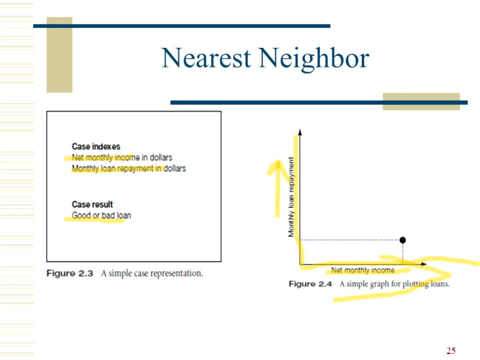 monthly loan repayment on the y-axis, And every case, let's say for this case, it has a certain net monthly income and a certain loan repayment. We can plot it on this 2D scale. That's quite easy, It's very simple. 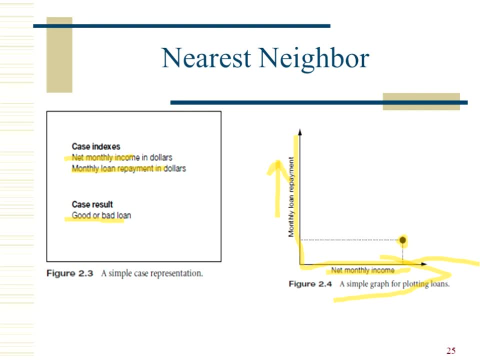 We can just take all the values for all the cases and we can plot them on this 2D scale, because we have only two features. We have two features: One can be labeled on the x-axis and the other one can be put on the y-axis. 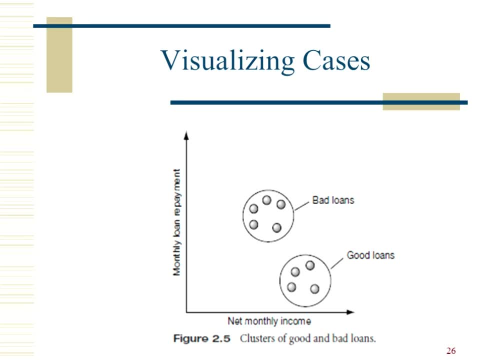 So if you try to visualize the cases, let's say we have put all the cases in this 2D space and let's assume that these are the bad loans, This cluster, it represents the customers who are not able to pay back their loan. 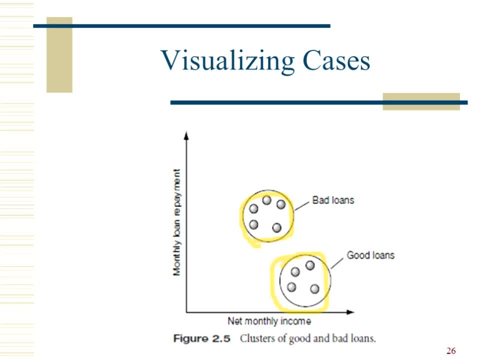 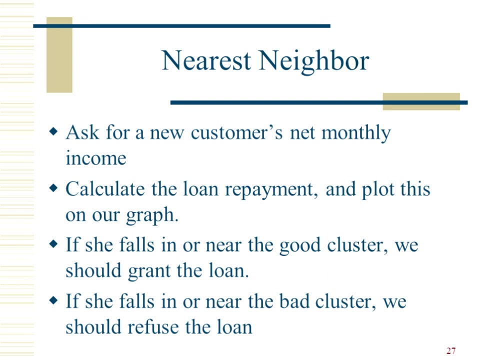 And, on the other hand, this cluster. it represents all the good loans. It means the customers, the set of customers, the customers in this cluster. all of them were able to pay back their loans. Now, when a new case comes, we ask for the customer's net monthly income. 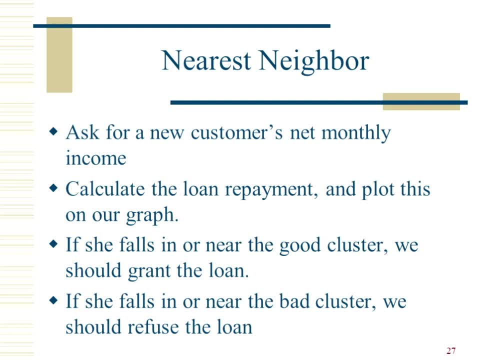 and we calculate loan repayment. Let's say, if the customer has taken, let's say, R100,000, and he is going to pay back in, let's say, 20 months, then the monthly repayment is, let's say, R100,000. 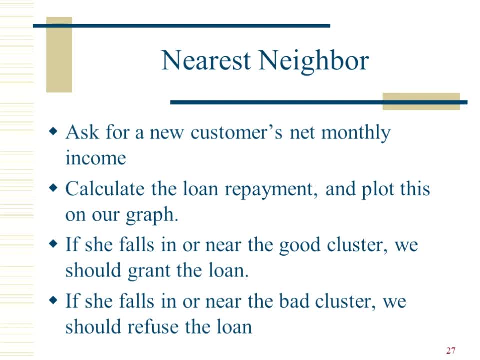 So we can calculate loan repayment. So now we can plot this on our graph. We have only two axes: the net monthly income and monthly loan repayment. We plot the new customer and if the new customer falls closer to the good cluster then we grant the loan. 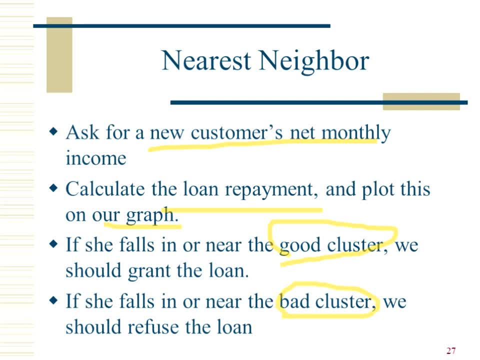 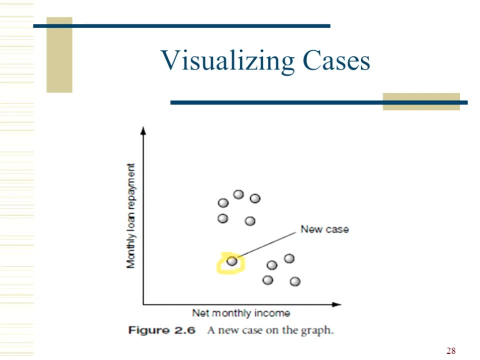 and if the customer falls closer to the bad cluster, then we refuse the loan. So here this is the new case. So we try to find the distance of this case or in fact, generally speaking, the similarity of this case with all the closest cases. 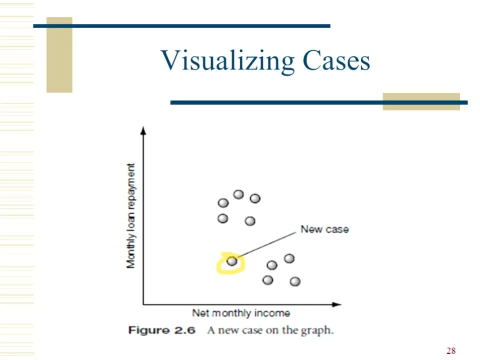 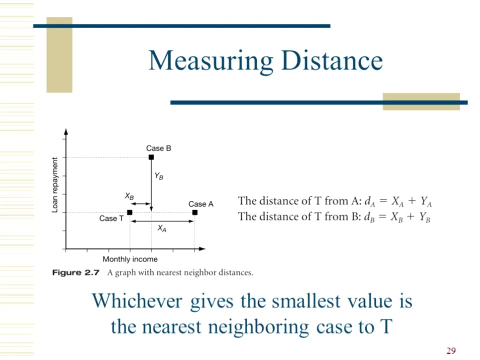 and then we see the solution. In this case, we see whether the closest guy to this guy was able to pay back the loan or wasn't Right. How do we do this? So here we are, using one technique. This is the Manhattan distance. 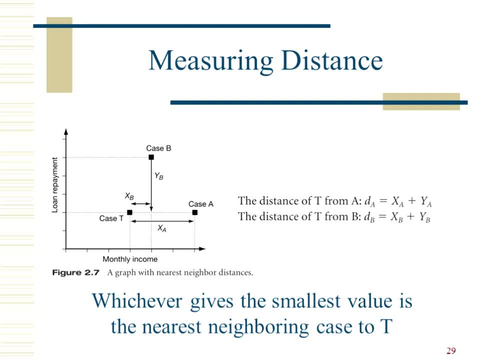 I hope you are aware of it. So what we do, we may have the. let's say, this is the new case. case T, it represents the new case and these two, they are the closest cases, case A and case B- Right. 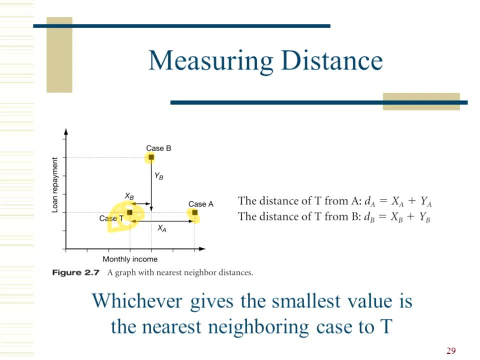 So what we do? we measure the distance in the x-axis and in the y-axis for both the cases and we add them up. So the distance of T from A is xA plus yA. What is xA? It is the distance in x-axis. 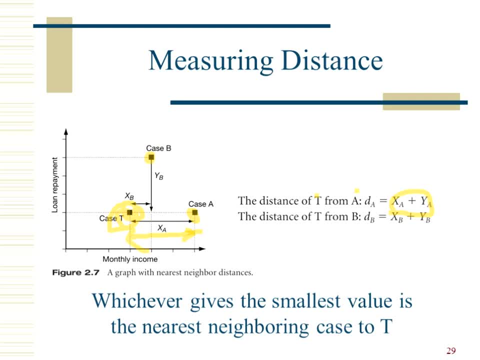 between case A and case T plus yA. What is yA? yA is the vertical distance between A and T. There is no vertical distance. They are in the same horizontal line. So this is zero. But whatever value we have, 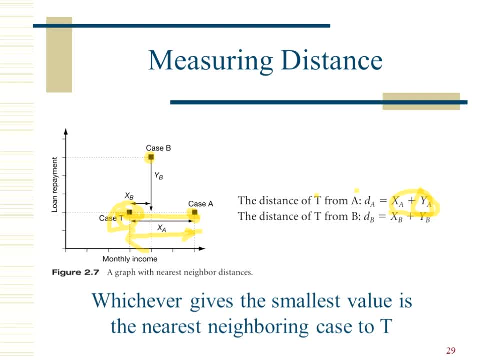 we'll put it here. If we put it here, this is zero, so it is not mentioned here. But in case of case B, this is the vertical distance, yB and xB is the horizontal distance, Right? So simply speaking. 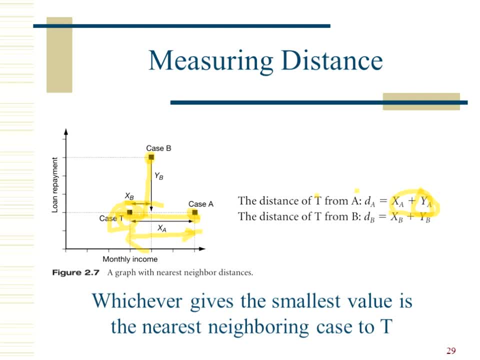 for the new case. we add up x and y, distance of the closest cases to this case. We add up both of them together and whichever gives a smaller value it is called the nearest neighbor to case T, And then we will see whether he was able to pay back. 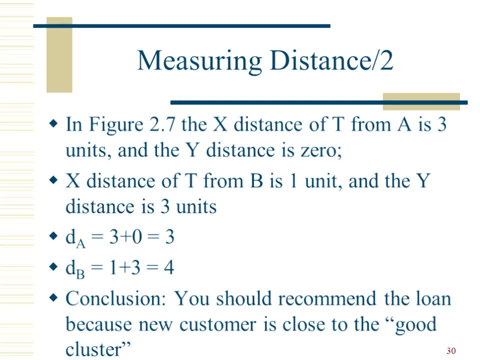 or he wasn't, And then we can predict that this customer will be able to pay back the loan or not. So let's assume in this figure the distance of the new case from A in the horizontal axis is three units and in the vertical axis 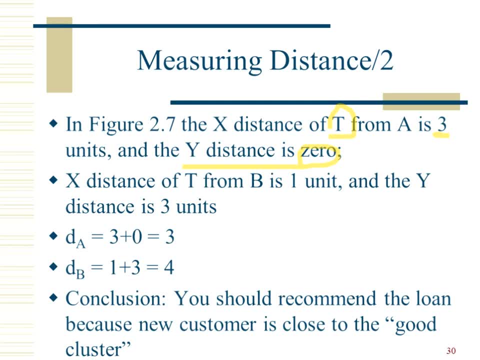 it is zero. They are on the same line. So the dA, can be said, can be calculated as three plus zero, which is three. And let's say the distance of this new case from B is one unit in x and three unit in y axis. 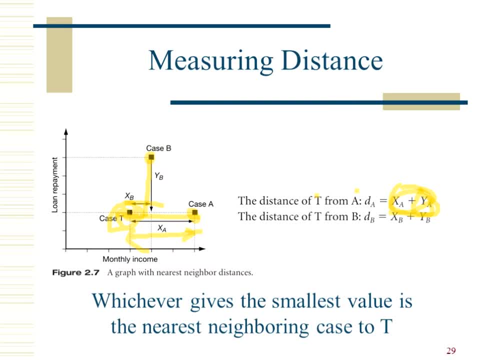 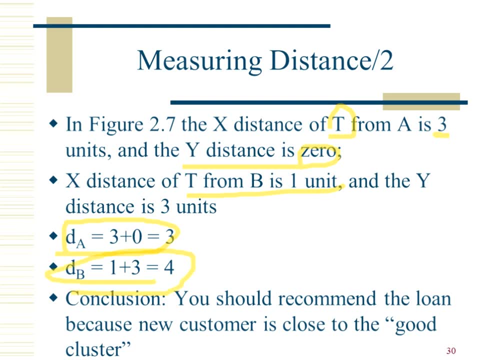 which you see here Here. Okay, One plus three, So this one comes out to be four. Right, So now we can say that the new case T, it is more closer to A, The distance is three as compared to B. 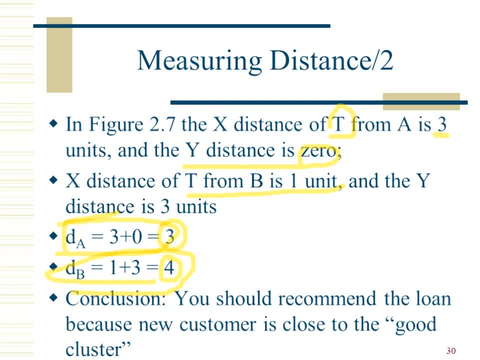 which is four, And let's say A belongs to the good cluster, So we can say that we should recommend the loan to be given to this customer, Because this new customer is closer to a good customer. It's closer to a customer who was able to pay back the loan. 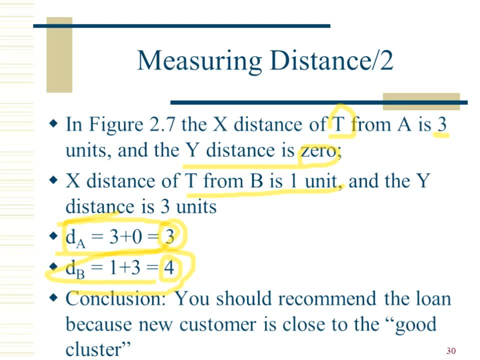 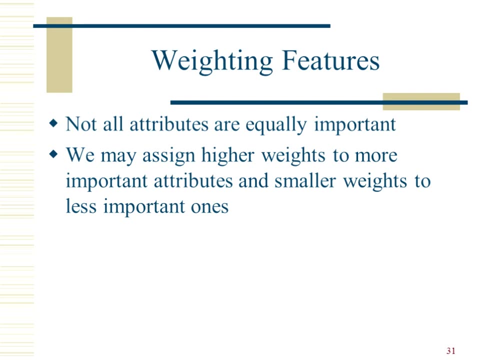 This situation: his monthly income and his monthly installments to repay. they are closer to this customer. He was able to pay back, so probably this customer will also be able to pay back The loan. There's also a waiting feature, a waiting scheme. 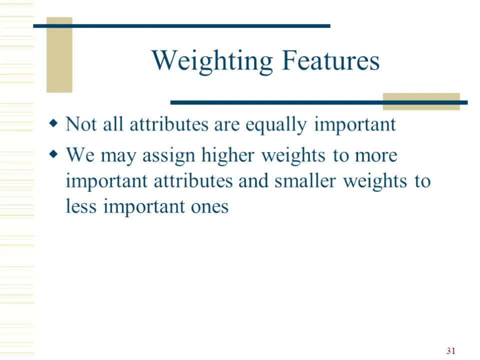 for the features or the attributes in the case space. The idea is that not all attributes are equally important. So in case space you may have some information which is more important as compared to some other information. So we can assign higher weight to the more important attributes. 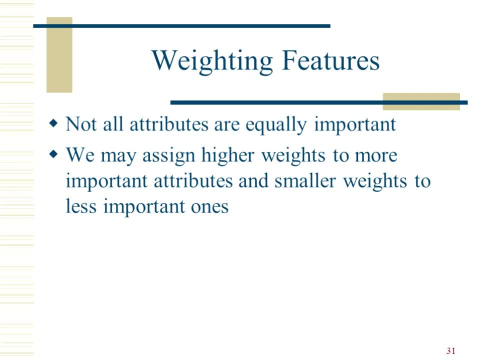 and we can assign smaller weight to less important ones. For example, for a patient, let's say, his or her temperature is important in diagnosis, but the MRI scan is more important. So we should assign more weight to MRI scan value or a blood test value. 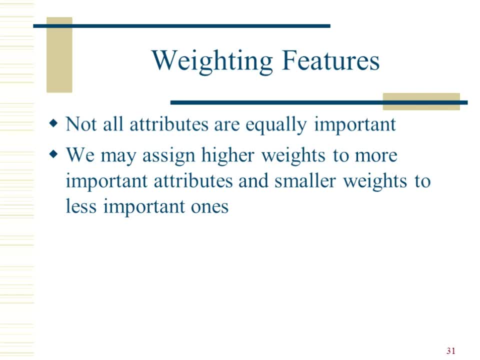 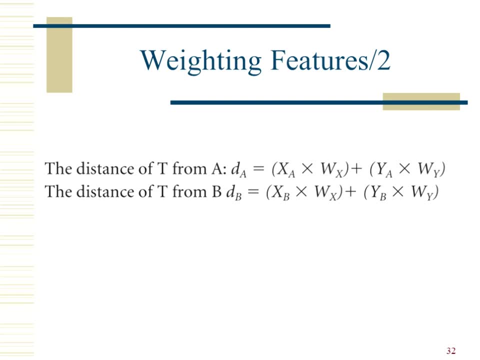 as compared to the temperature of that patient. So we can assign more weight to the features and then we'll multiply these weights with these features. So here we have only two features: xa and ya distances. So we can assign, let's say, 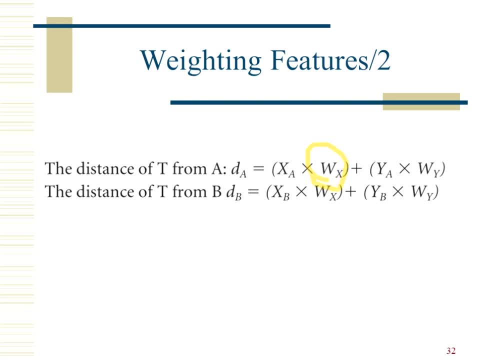 wx to the x-axis and wy to the y-axis. So now the distance formula will be revised as xa into wx, plus ya into wy, and same for the distance, The distance of case t from the case v. We just multiply the weights with those features. 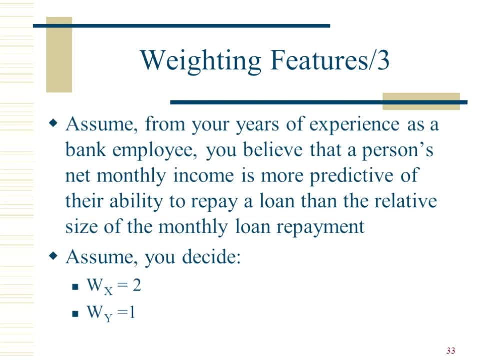 or attributes. So, for example, let's say, from your experience, from your vast experience, you believe that a person's net monthly income is more predictive of their ability to repay a loan than the relative size of monthly loan repayment. So let's assume that 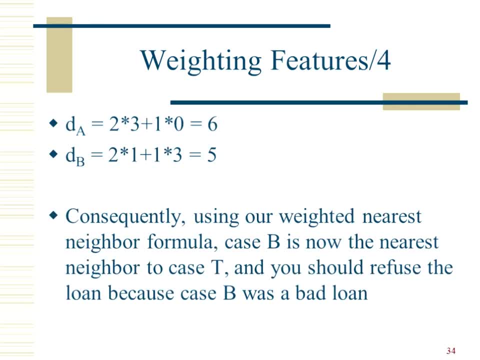 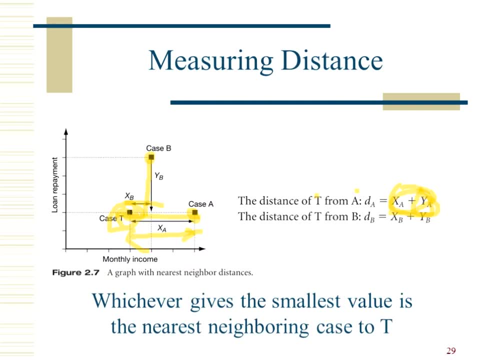 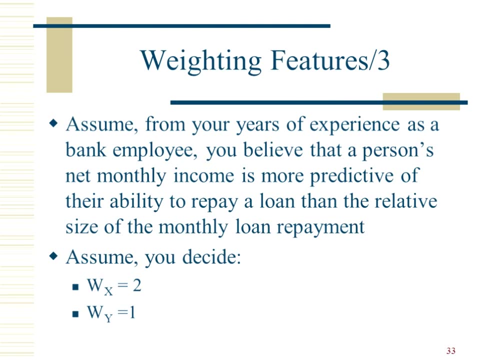 you believe that horizontal x-axis is more important than the y-axis. We have plotted. if we go back, yeah, monthly income is plotted on the x-axis, So this is more important than the y-axis. So we can assign, let's say, 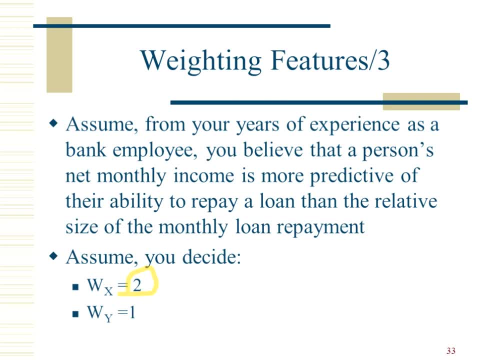 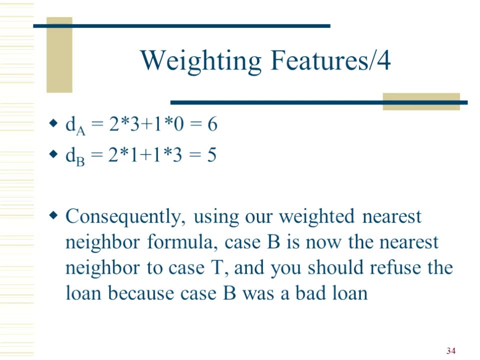 weight two to the x-axis and we can assign one to the y-axis. So if we use these weights, then now if we can calculate the distance of this case from case a and case b. now we multiply the x-axis with two and y with one. 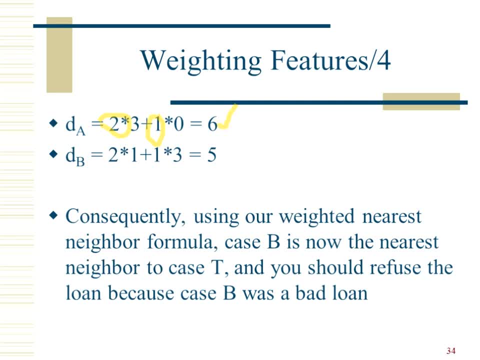 for both of them. And now the distance from case a is six and the distance from case b is five. And now this new case is closer to case b, And case b is a bad case. This guy was unable to pay back. So, based on this model, 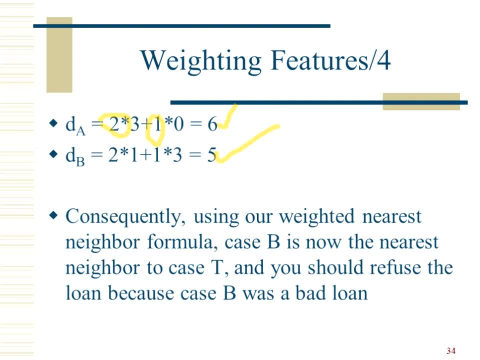 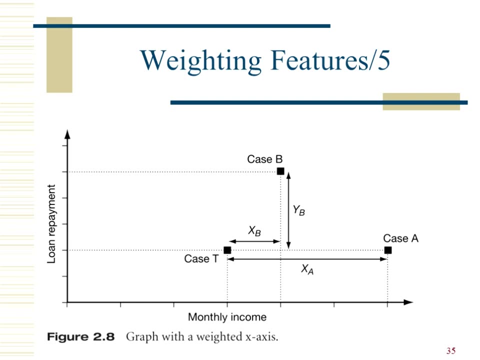 based on this setup, this formula, we can say that we should not recommend loans to this new customer because he is more closer to the bad cluster. Another way of looking at it is like we have extended the x-axis by two times, So visually also. 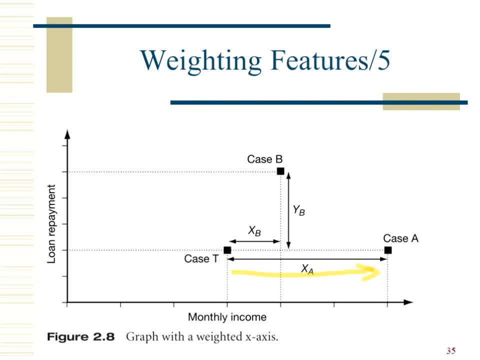 you can see, previously this value was three, but now it is six, and by naked eye you can also see that this case is closer to case b as compared to case a, right. So this is one way of looking at it in which we have a graph. 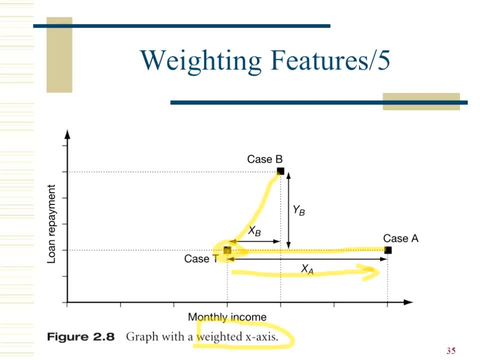 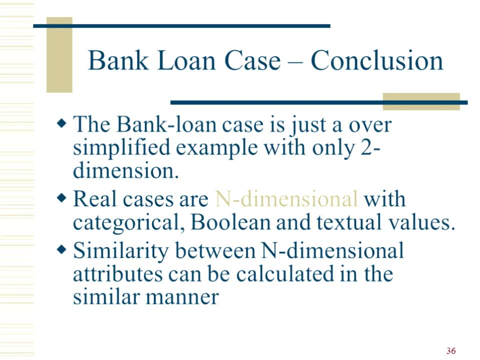 with the weighted x-axis. And here it is just for the real aspect. Of course, mathematically it doesn't have any implication. So to conclude, this bank case is just an over-centrified example with only two dimensions We just talked about. 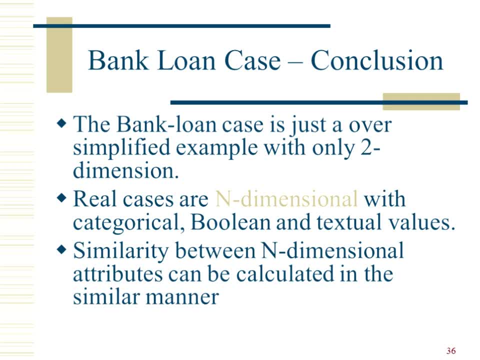 two dimensions: the net monthly income and the monthly installment to pay back. But in any real life scenario we will have n-dimensional cases. We may have 10, 15,, 20,, 30 or even hundreds of attributes to describe a case. 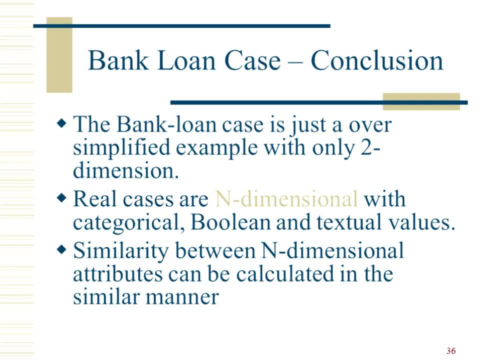 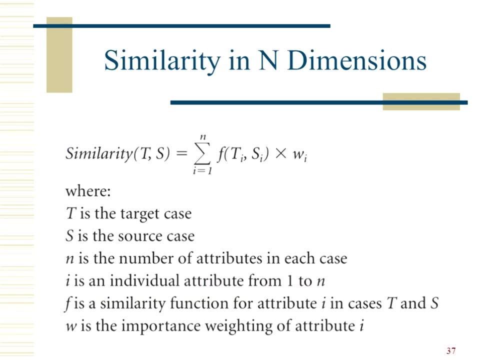 and we may have the category of values. we may have Boolean values, we may have textual values, We can have a variety of variables. So similarity between n-dimensional attributes can be calculated in the similar manner, just like we did for two-dimensional. We can extrapolate it. 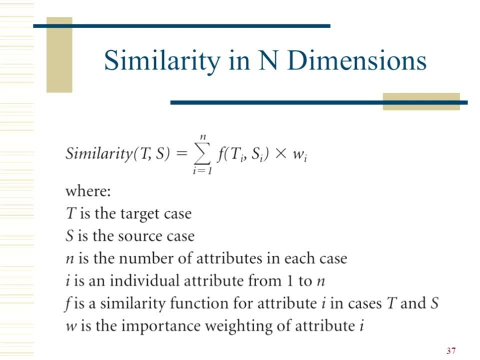 to n dimensions. So we can say that similarity of a new case t with an existing case s is a sum of this. sum of what? Sum of n values? What are n values? These are the number of features, and for every feature we have f and w. 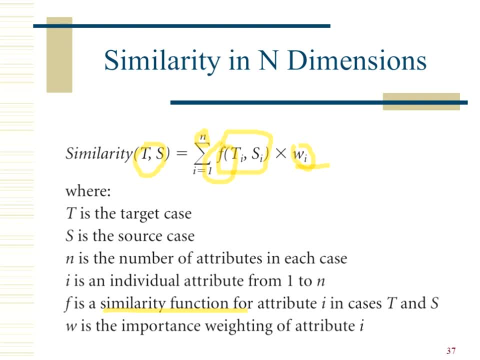 What is f? f is the similarity function and w is the weight. So to find a similarity between new case t and an existing case s, we will add up similarity multiplied by weight of all the features in that case Right And similarity functions. 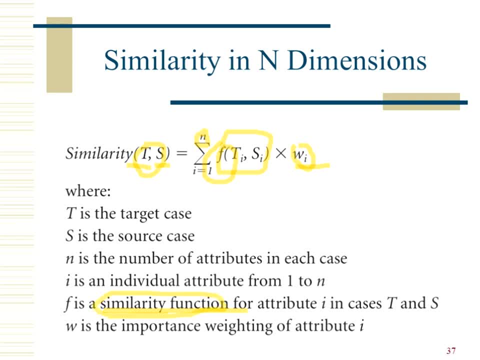 can be different, Like in this case of the bank loan. we were taking the Manhattan distance. We may also take the Euclidean distance. We have discussed in advanced information system that co-signs similarity measure Right. There can be many ways in which we can find. 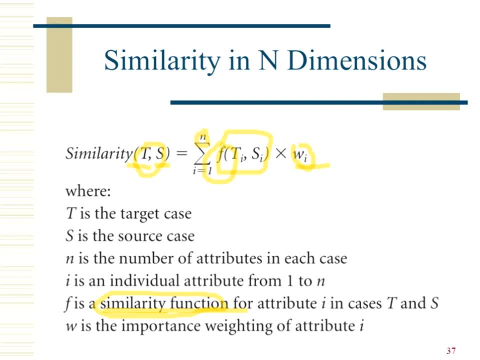 a similarity between the two attributes, But we will have a similarity function and we will have a weight of that feature. Just multiply all the features, all the functions, with the respective weights and add all of them and you will get a final value for similarity between. 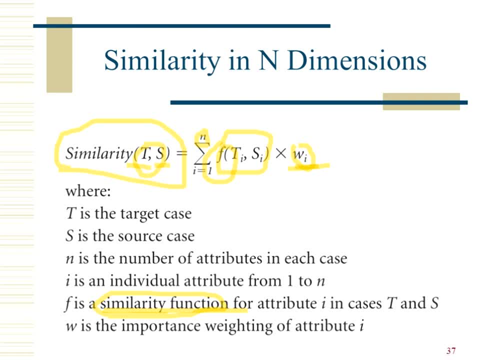 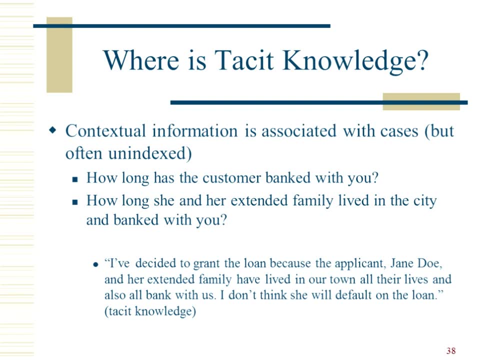 this test, new test case and existing test case: Right? So it was a very basic explanation to tell you how we can find similarity or how we can retrieve the relevant cases. But one thing may come to your mind, that where is the tested knowledge? 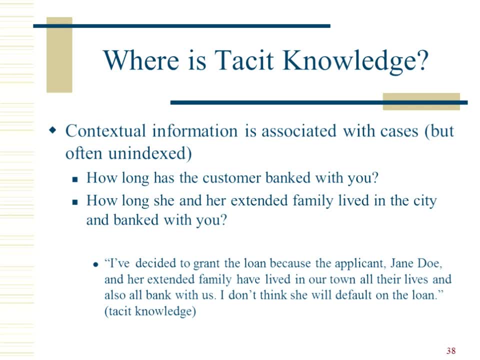 It was all explicit, but we discussed in the beginning that the tested knowledge also needs to be considered. Well, the tested knowledge is there. We need to associate it with the cases. However, it is not in-depth. It is often un-indexed. 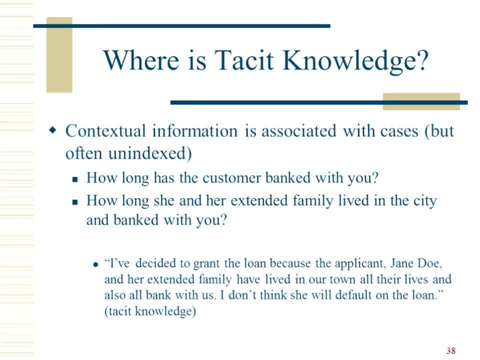 You know about the tested knowledge. It is not easy to index, So in this case, just to tell you how the tested knowledge can be used, let's say, in this case, the bank manager. he knows how long has the customer banked with him, or the customer's. 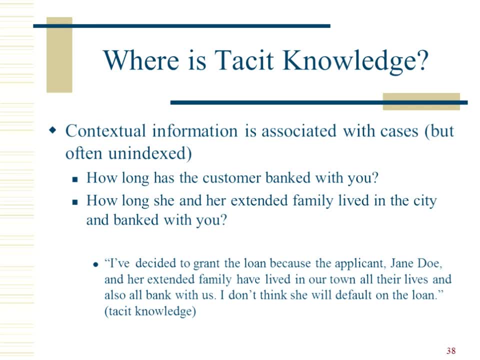 extended family their loyalty with the bank also. if you have this information, So you may say that I decided to grant the loan because the applicant and our extended family have lived in the bank for a very long time and the bank has been in the bank for a very long time. 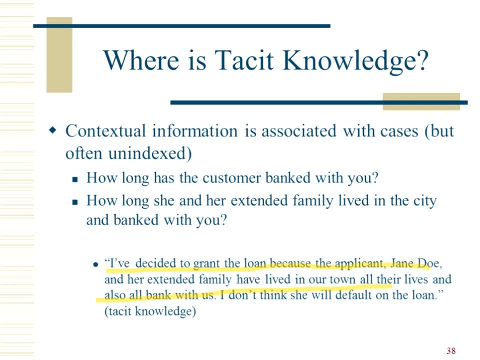 and the bank has been in the town all their lives and also all of them. they bank with us. I don't think that she will default on the loan. So you can use the tested knowledge like you can override the solution, and you can by using 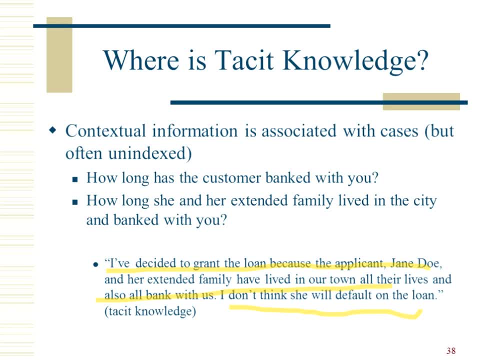 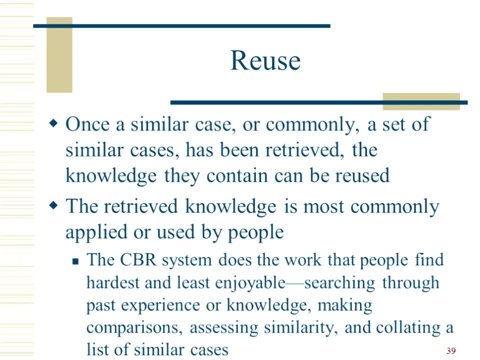 tested knowledge, you can come up with a new solution. So this is one way of using tested knowledge. in the CBR We use the second chapter, we use the solution. in the other cases they have been retrieved. the knowledge they contain can be reused. We reuse 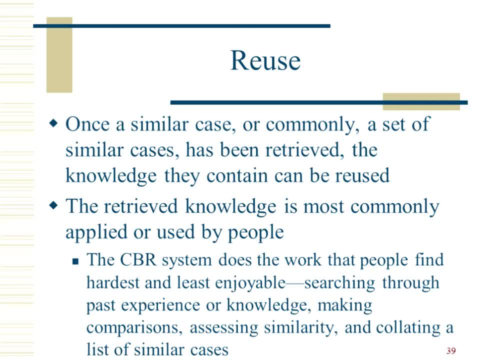 those solutions, just like we did in this case. So the retrieved knowledge is most commonly applied or used by people, Most of the people that use it. The CBR system does the work that people find hard and enjoyable, So the CBR system will. 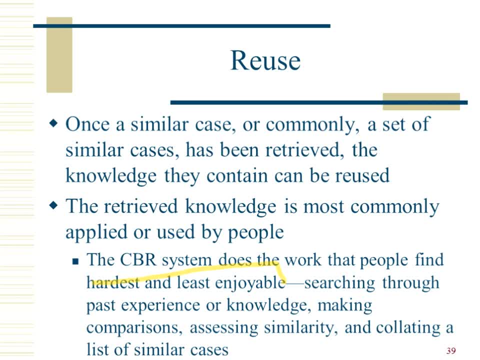 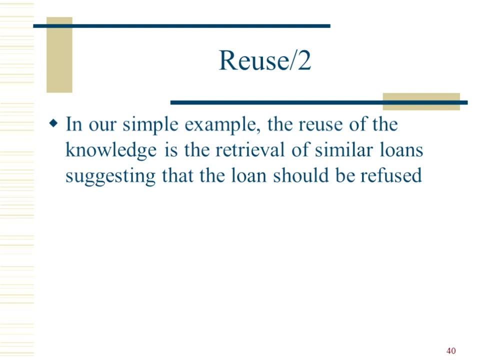 use, which is hard for the users. it is done by the CBR, but ultimately the reuse will be done by the people and they will also use the artistic knowledge to solve the new problem. So in our simple example, the reuse of knowledge is the retrieval of things, suggesting that 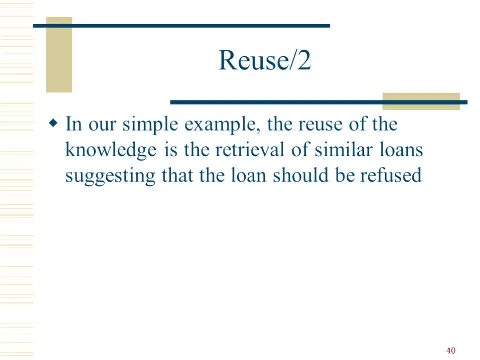 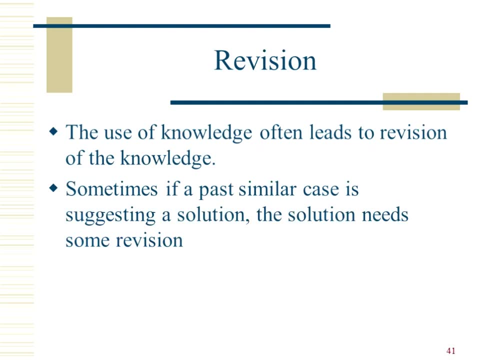 the loan should be refused in the second model or it should be granted in the first model that we have used without using weights of the feature. Next is revise. The third step is to revise the solution. The use of knowledge often leads to revision of the knowledge. 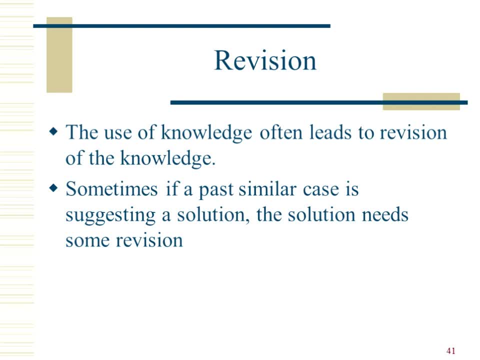 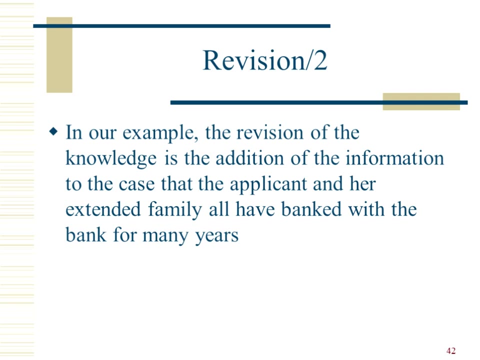 Sometimes in the past, in the case of just a solution, the solution needs some revision. You need to tweak the solution to solve the new problem, For example, in our example we have a solution, For example, of bank loan. the revision was that the bank manager considers the loyalty. 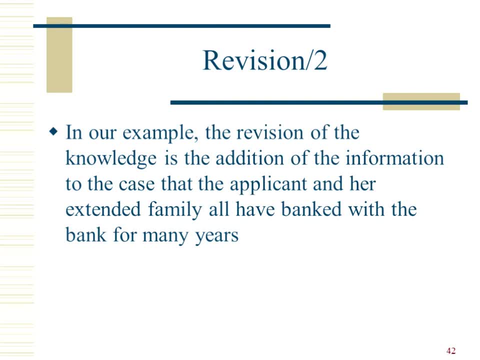 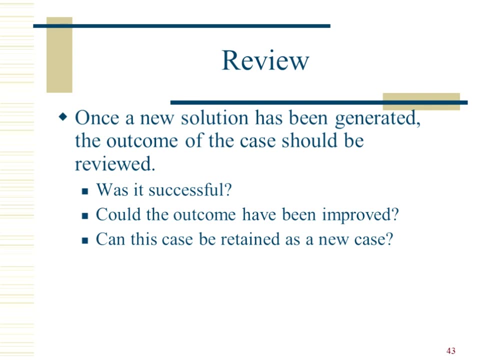 of the customer and their relationship with the bank, and then overrides the solution, revises it to recommend the loan to this customer. Next is review. Once an new solution has been generated, the outcome of the case should be reviewed. So we have proposed an new solution and now we can review it to see whether or not the 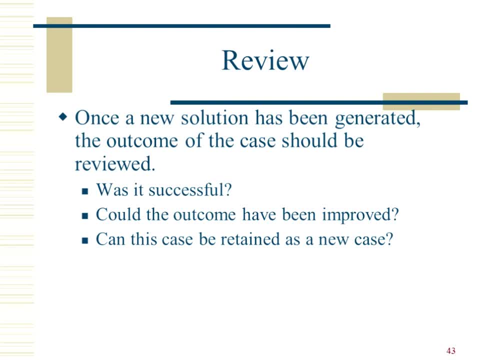 solution was successful or not, because then it will become a part of the case base and it will help in solving the other problems in future. We can also review how the outcome could have been improved or can the case be retained as a new tool. 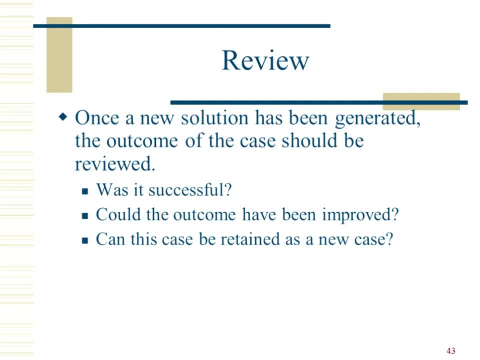 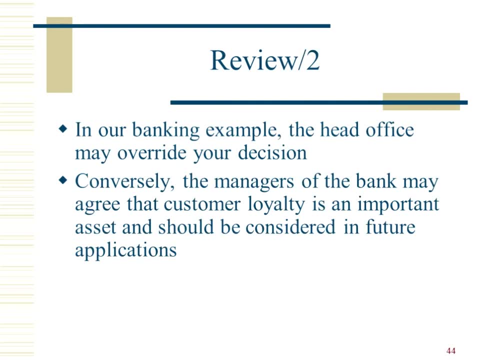 Does it add any new information, any new knowledge which is not already there in the case base? So we can review the case base Now, banking example: the head office may override your decision. That's it. When you make a recommendation as a bank manager, the head office may say that, okay, this justification. 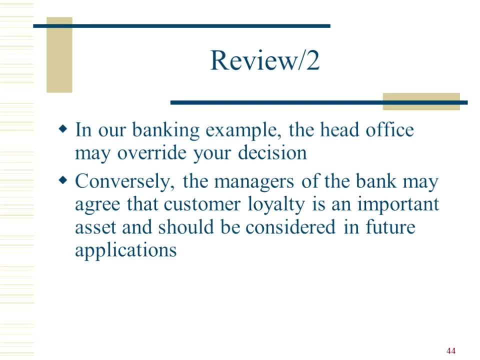 is not valid. Even if the customer is a loyal customer, this loyalty should not be considered in making the decision. They may override, Or they may also agree with you and they say that, okay, customer loyalty is an important feature and it should be considered in the application in future. 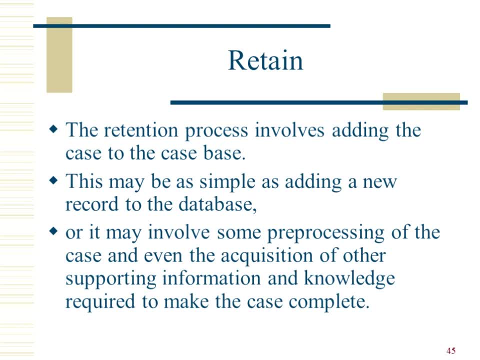 Next, we'll retain the review. The retention process involves adding the case to the case base, so now this new solution should be retained in the case base. It will help in solving the problems in future. It can be as simple as adding a new record to the database, just like we add a record. 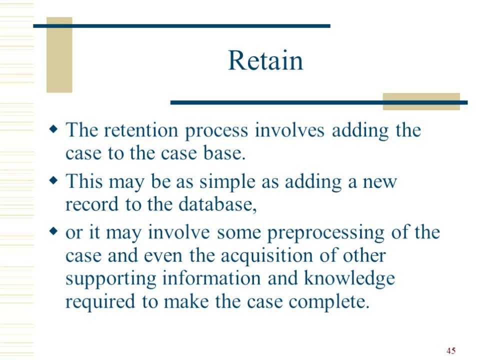 to the database. We can just add a case in the case base, or it may involve some preprocessing of the case and even the acquisition of further supporting information and knowledge required to make the case complete. We may have any supporting information, Just like the case. 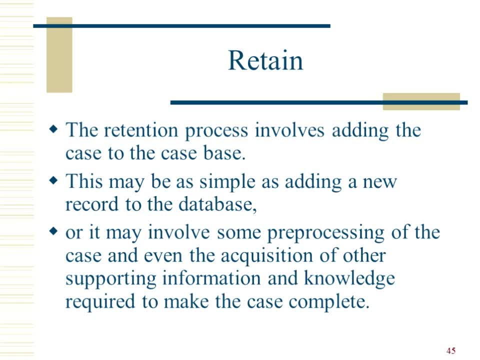 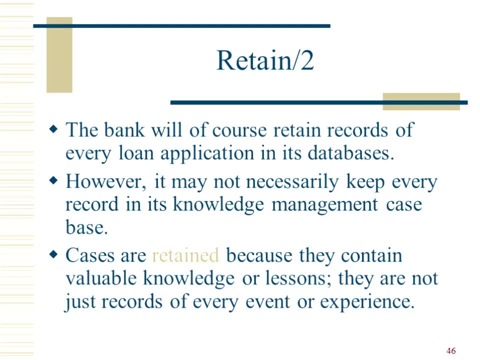 In this case, the managers use the loyalty aspect of the customers, so we may capture this information to make the case complete. The bank will, of course, retain the records of every loan application in its database. However, it may not necessarily keep every record in its knowledge management case base. 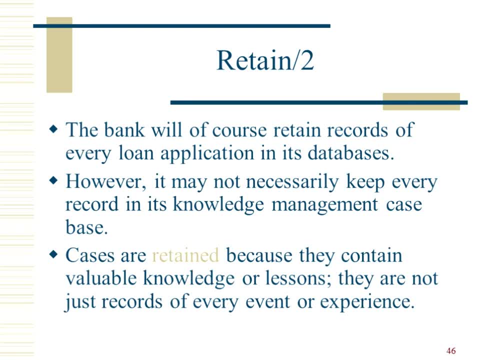 So we put all the customer applications and decisions in the database, but it might be useful to put every case, every application in the case base as well. Cases are, again, because they contain valuable knowledge or lessons. they are not just records of every event or experience. so they should add some value to the case base. 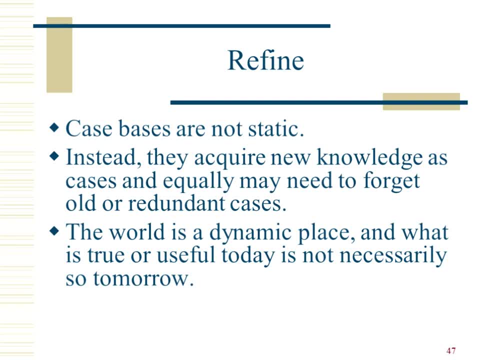 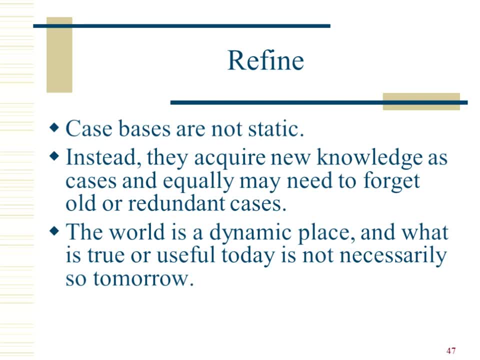 The last step in the CBR is to refine the case base. The case base is not a static thing. Instead, they acquire new knowledge as cases and equally may need to forget old or redundant cases, So we always need to keep updating our case base. 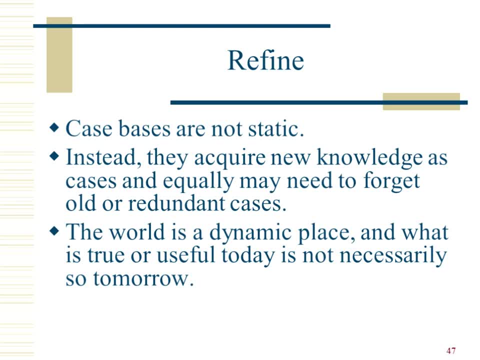 If we have any redundant information, we should delete them, we should forget them, we should discard them from our case base. What is a dynamic place? and what is true or useful today is not necessarily true tomorrow. So we may have collected some information. 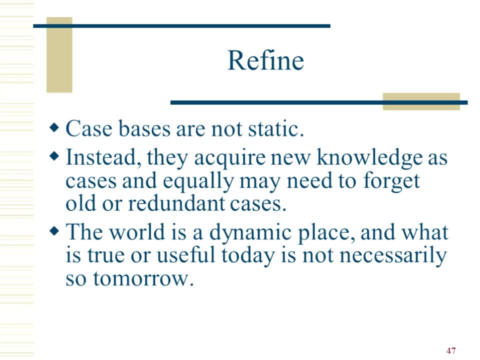 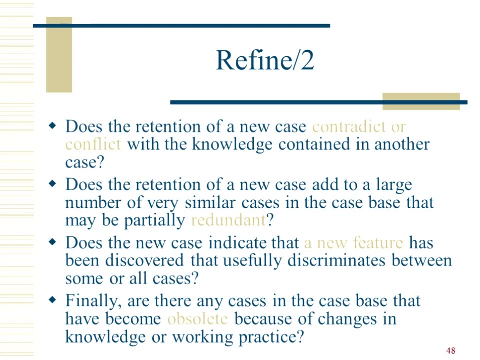 We may have collected some information five years ago and today maybe things have changed dramatically, So we may need to prune our case base. we may need to delete those case bases. with constant review. There are many questions we need to ask whenever we are refining our case base. like: does the? 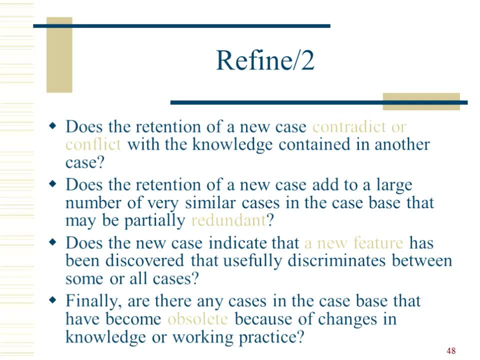 retention of a new case contradict or conflict with the knowledge contained in another case. So whenever we are adding a new case, we need to ask ourselves: is it consistent with the other cases or it contradicts with some previous cases? Does the retention of a new case add to a large number of very similar cases in the